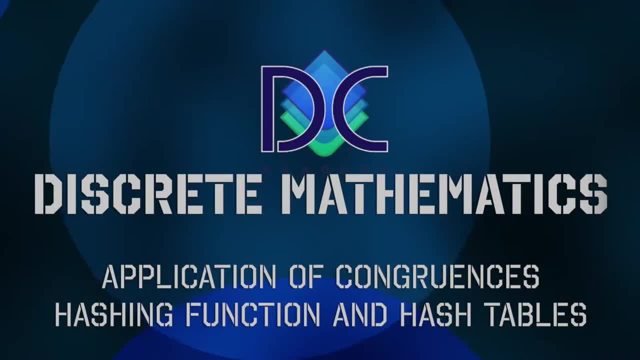 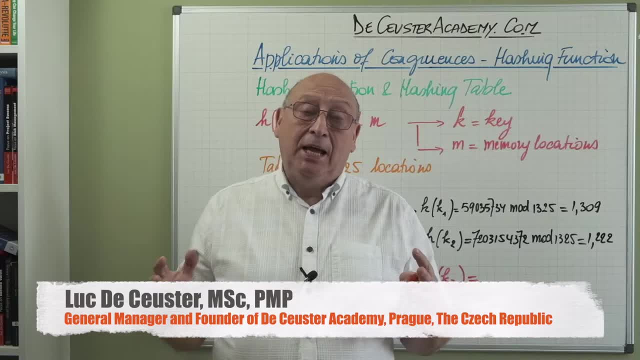 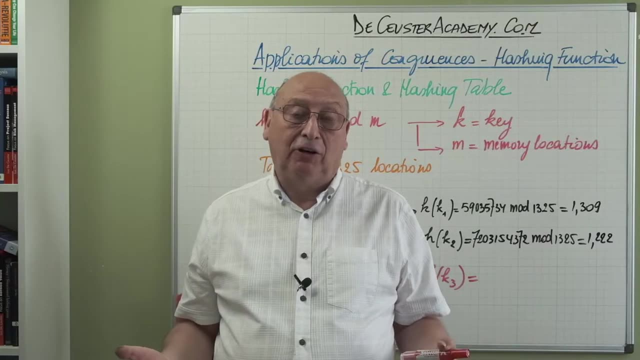 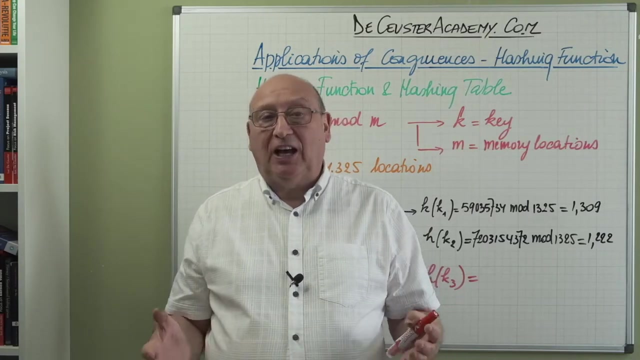 Great to see you here again in this new video offered to you by the Koster Academy. My name is Luc de Koster and I will be presenting you a new video about hashing and the hashing function, which are, in fact, applications of congruences. But before we start, do not forget to click the. 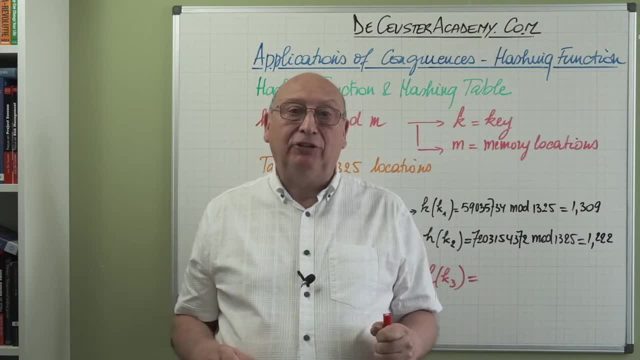 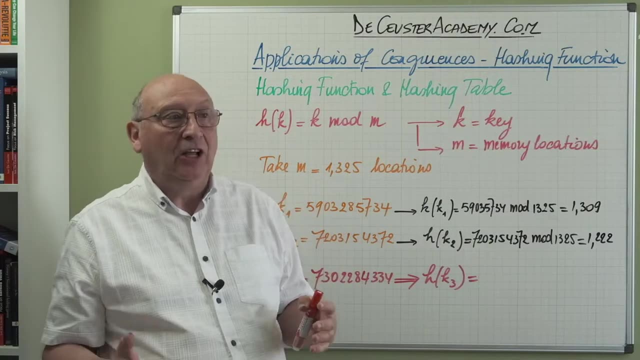 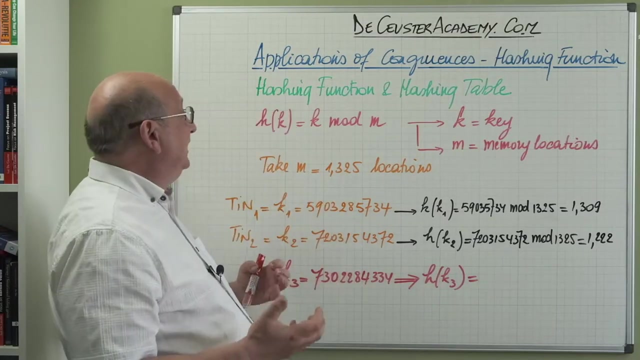 subscribe button, click the bell button, and every time we have a new video, you will be informed. Now, we've been using congruences, we've been defining modular arithmetic. for some reason, of course, we want to do something with it, And one of the things that we are going to use is hashing. 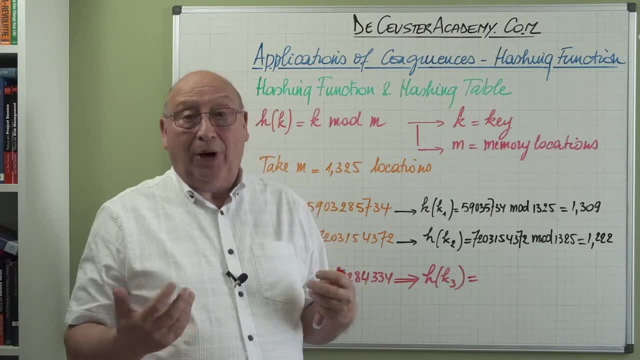 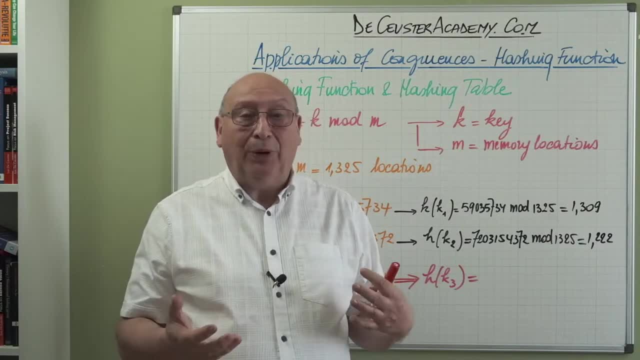 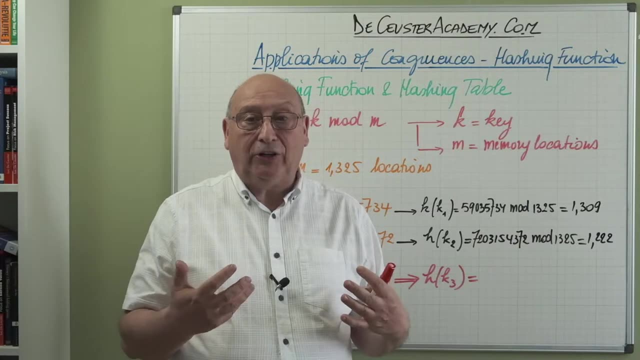 since this is a very large number. since this is a very large number, since the amount of data is always the amount of data is always increasing and we want to find some data in the computer, we basically have to go and conduct brute-force algorithms like linear search, to go through. 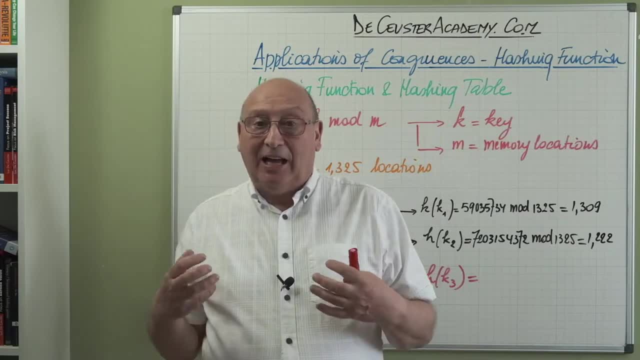 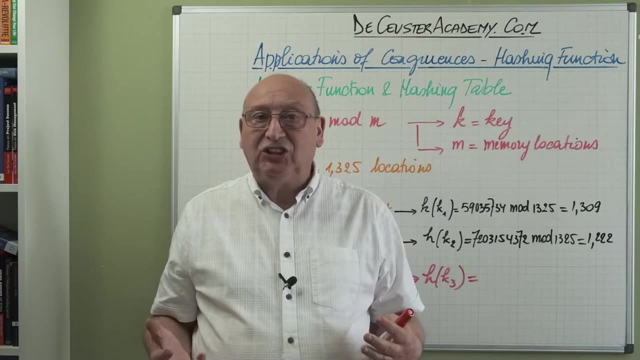 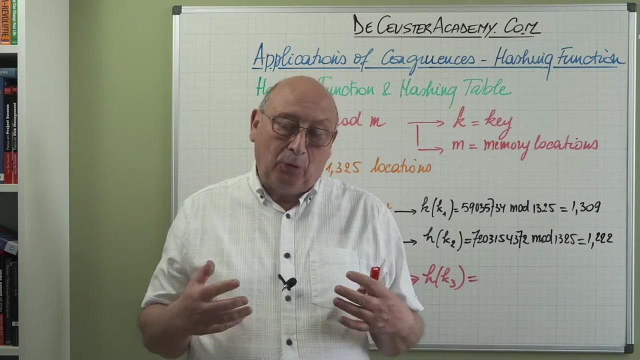 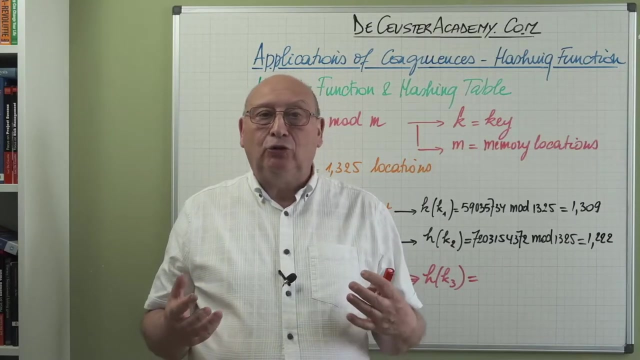 every space, every allocation of memory that contains data, to find the data- And that's not really very interesting because the search time would be very high and we want to avoid that When we introduce the hashing function and create the hash table. basically, what we're going to do, we're going to use modular arithmetic to allocate a memory space. 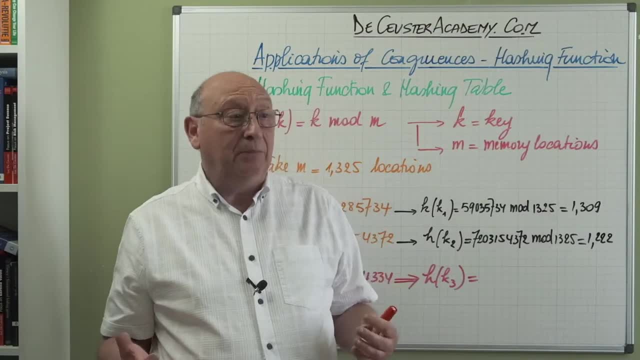 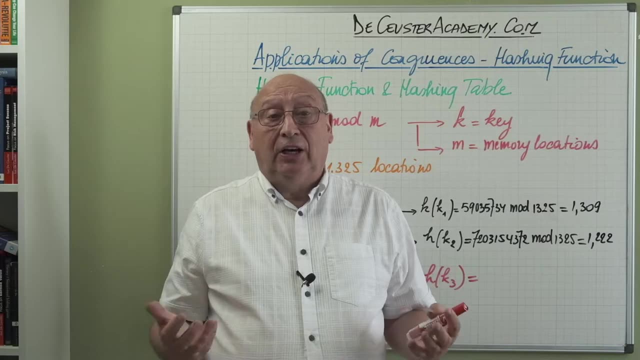 to a specific number And these numbers can be telephone numbers. they can be the personal numbers, like we have in Czech Republic or other countries. there can be the tax identification number. they can be the personal numbers, like we have in the Czech Republic or other countries. 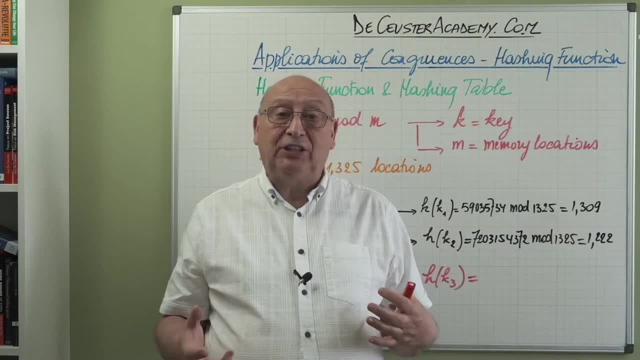 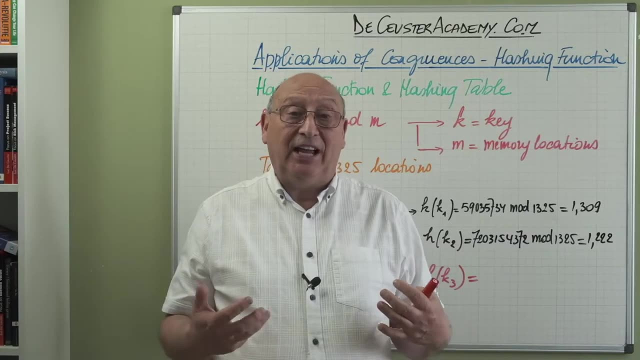 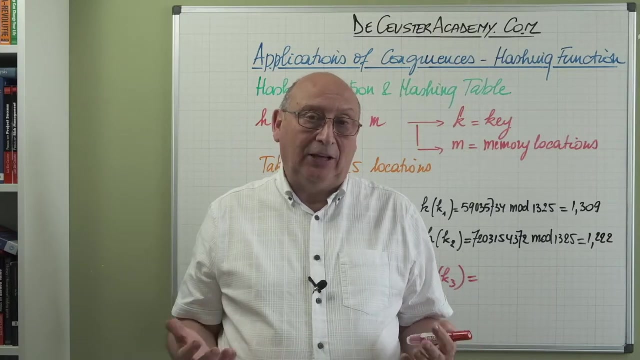 there can be the social security number. All these numbers can be in fact stored. even strings can be stored, because in the computer, every letter, every symbol, even a space, has a numeric code, ASCII code. we can use those, but let's start just with numbers. Now a hashing function. 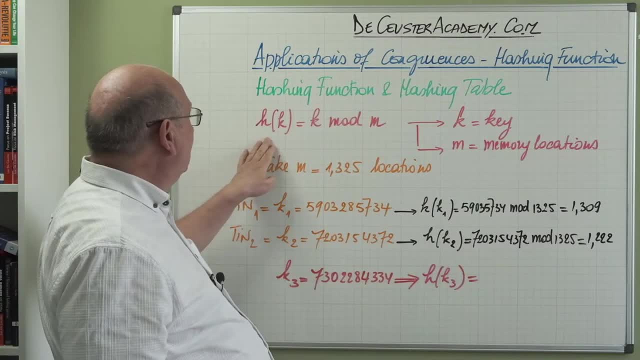 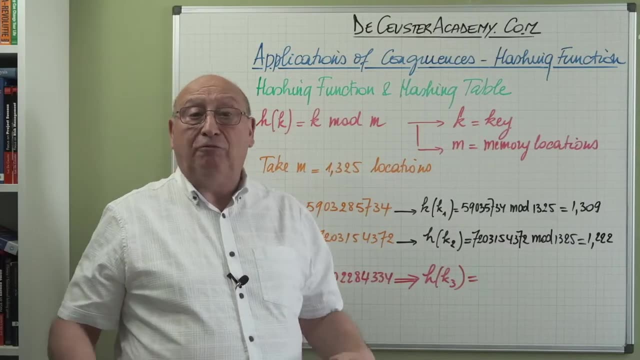 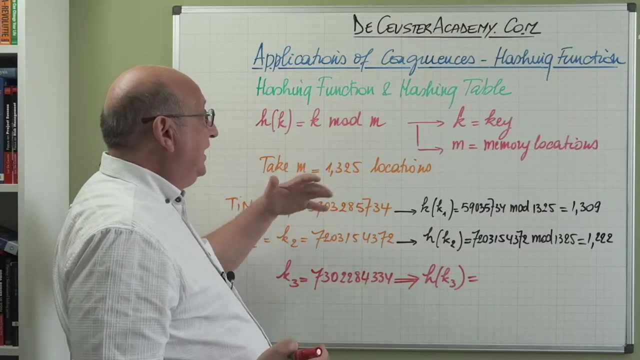 and a simple hashing function is a function like this: h of k is k modulus n, So k is the key and M is the amount of memory locations that are available. now, what are we going to do? we're going to find the key. we have a numeric value in our 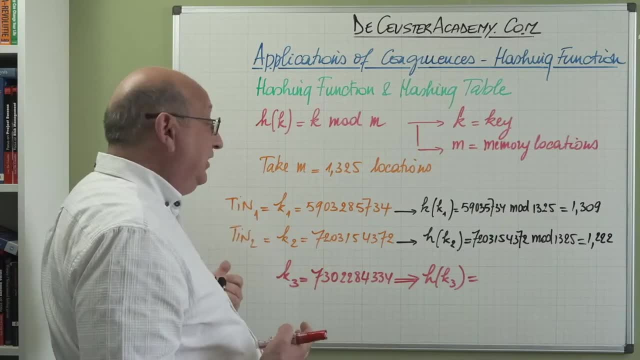 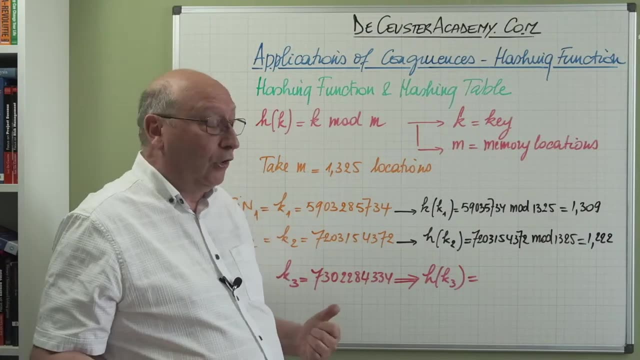 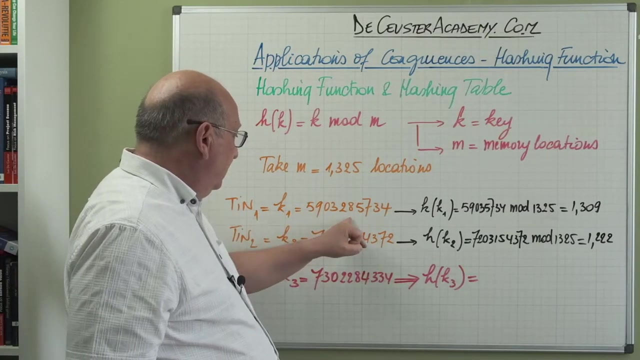 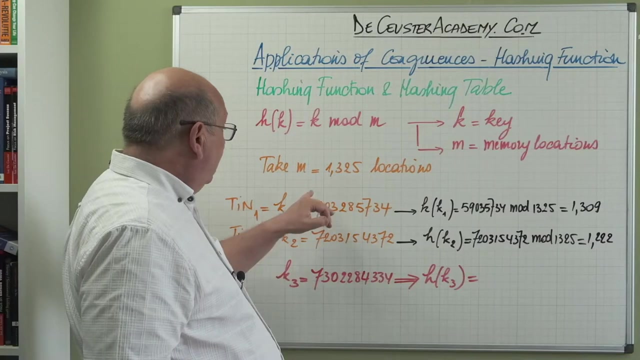 case, we use a tax identification number which is a little bit similar, like the personal numbers that we know in several European countries, which is composed first of the birthday, starting from the year till the day, and then a number which is basically unique for every individual. we have to see what are the 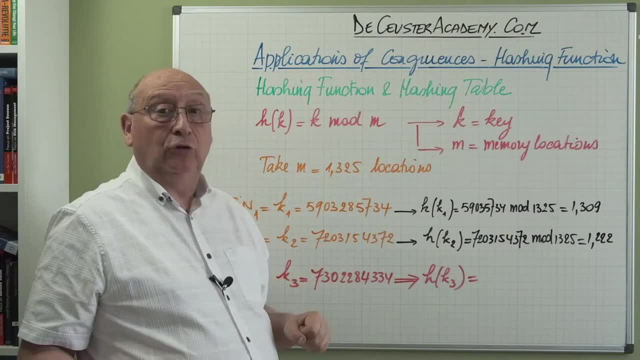 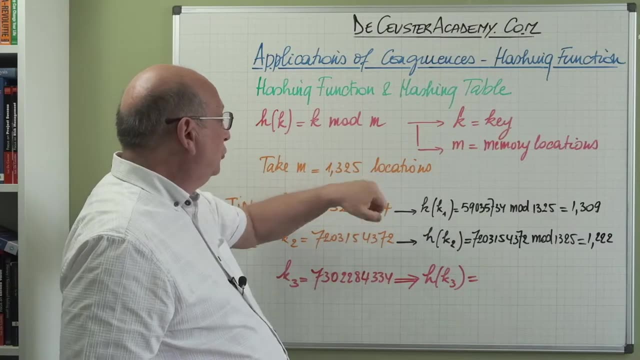 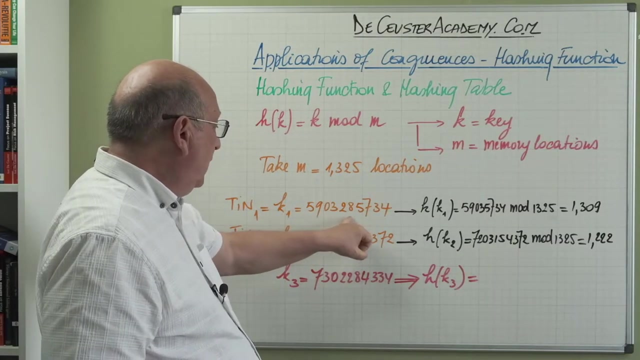 locations. we have, in our case, 1325 locations and we are going to apply the hash function K modulus M, K modulus 1325, and our first number, K1, is 5, 9, 0, three, two, eight, five, seven, three, four, and when I use the hashing function, I: 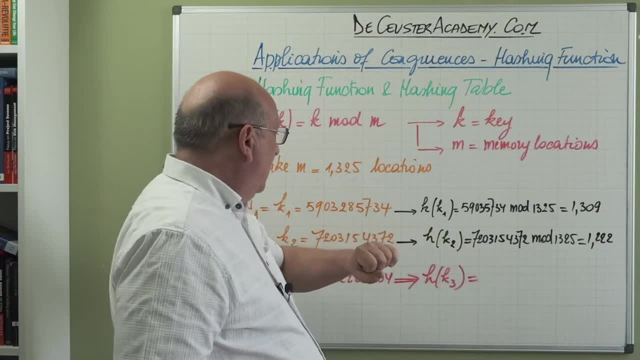 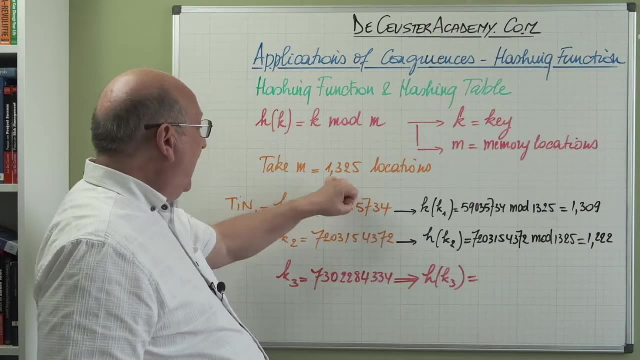 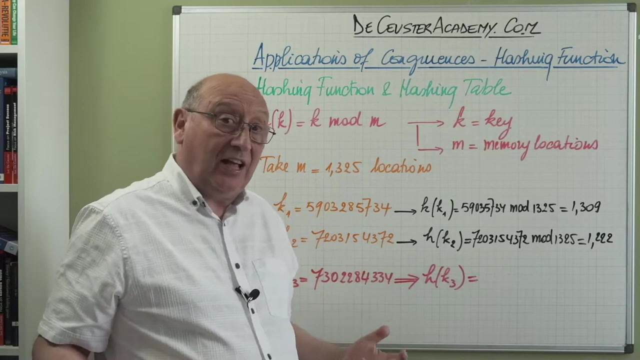 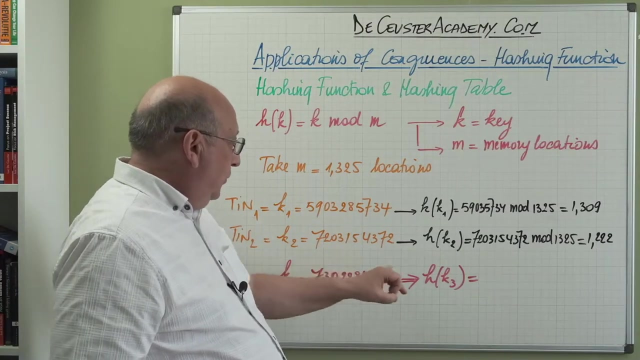 find in fact that the model is that fifty nine zero three, two, eight, five, seven, three four, divided by one thousand three hundred and twenty five, has a remainder of one thousand three hundred and nine. we can calculate that your masters added by now. we can do the same for the second one, but here we 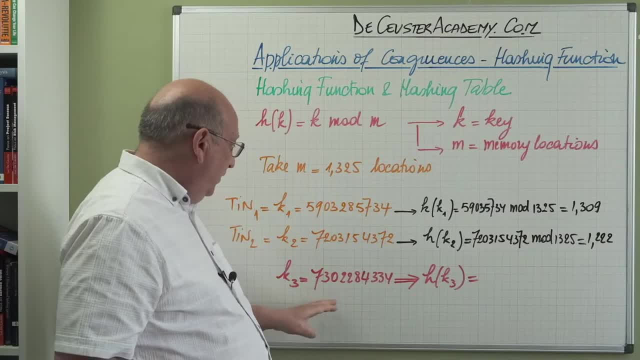 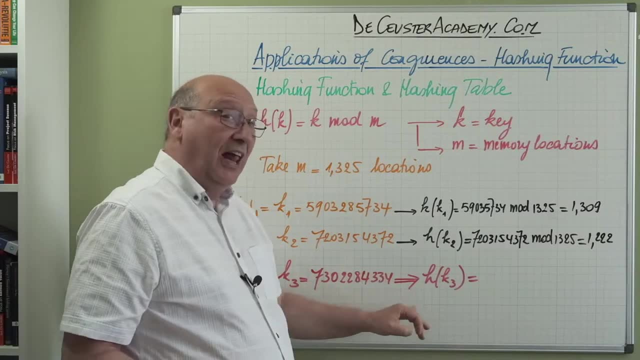 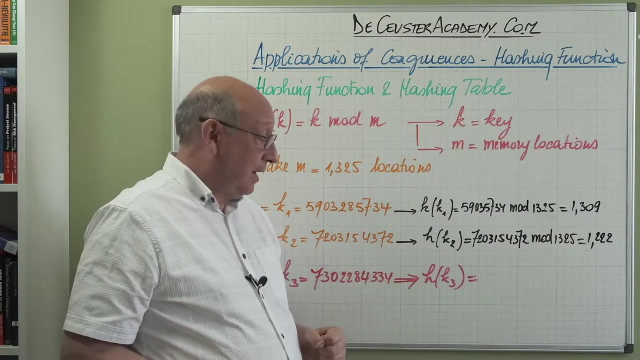 find 1222, and let's have another number here: k3. try to calculate the value of the hashing function. just stop the video and see what happens next. so you're back. you did the calculations or you didn't do them. it's not a problem, you can review. 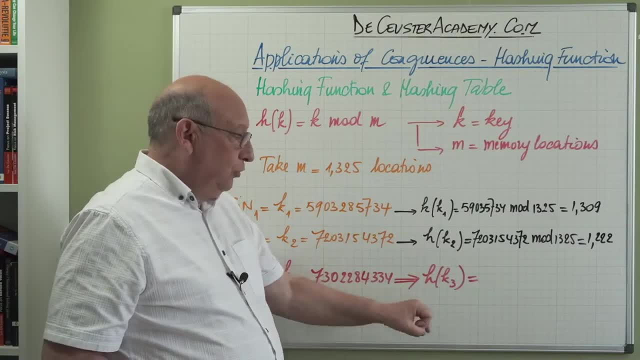 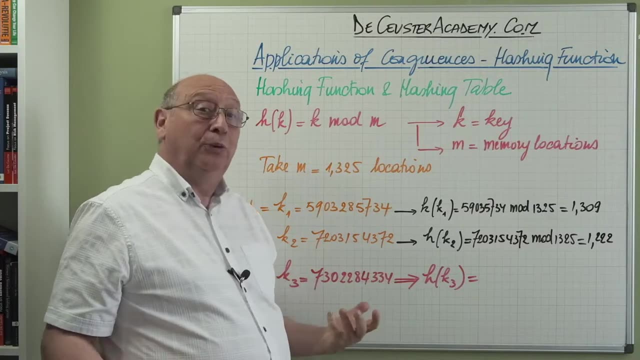 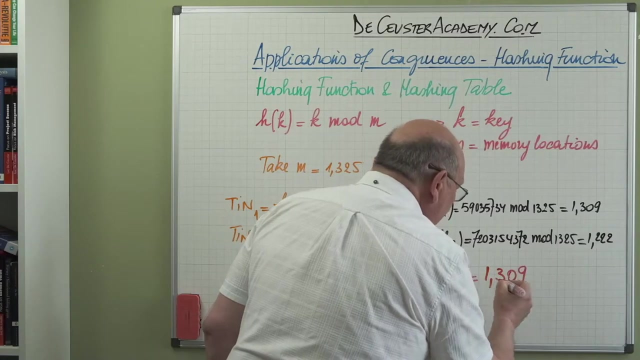 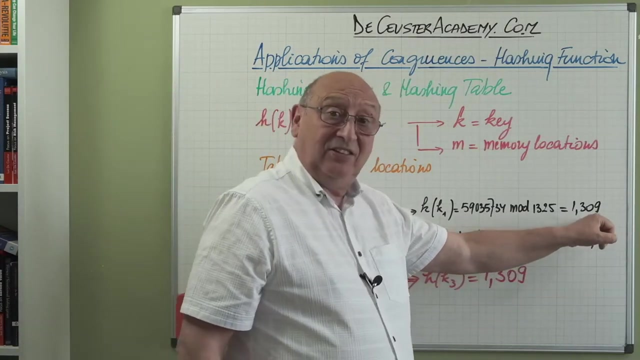 it later. you can have other examples. when we do, when we apply the hashing function. I'm this new key. what do we find? we find that the memory location 1309 is allocated to this new key. but what do we see? we see that this memory allocation. 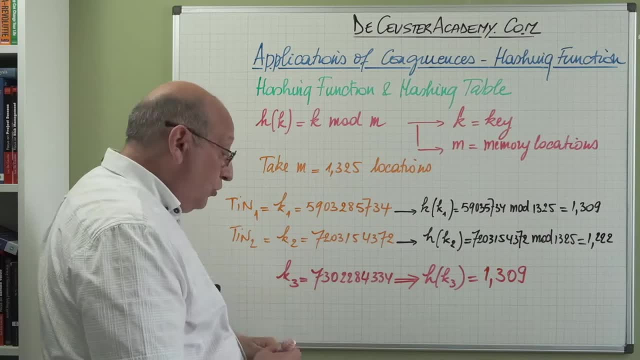 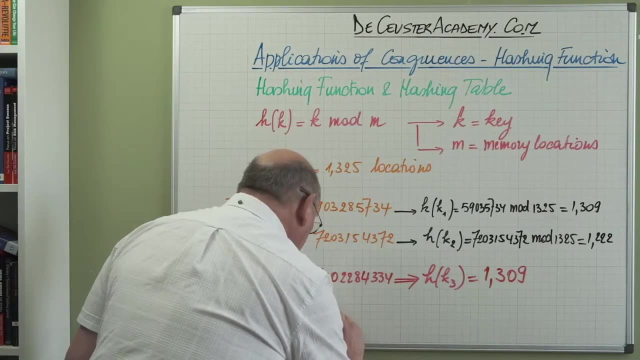 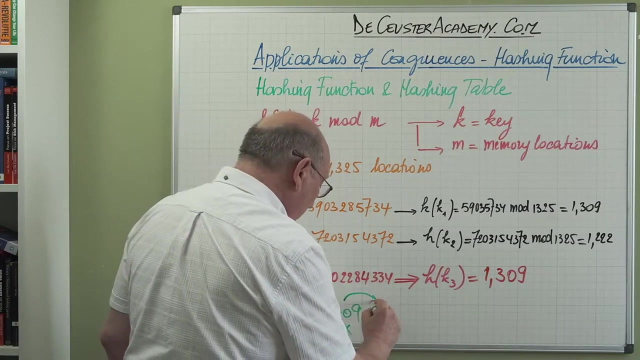 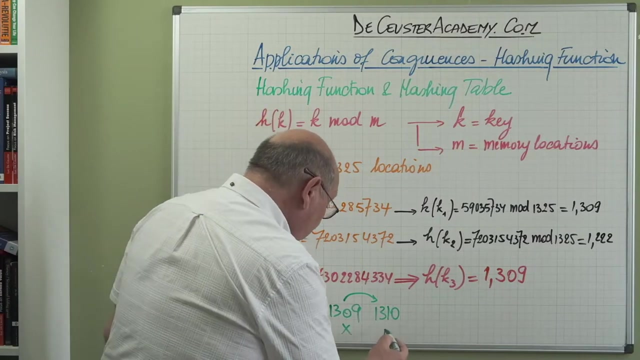 has already been used. so basically, when we go to the memory, we see 109, one thousand 309, which is full. what we do now is we go just to the next one, 1310. is this free, yes or no? then we say, okay, we will put it there, but if it's not free, we. 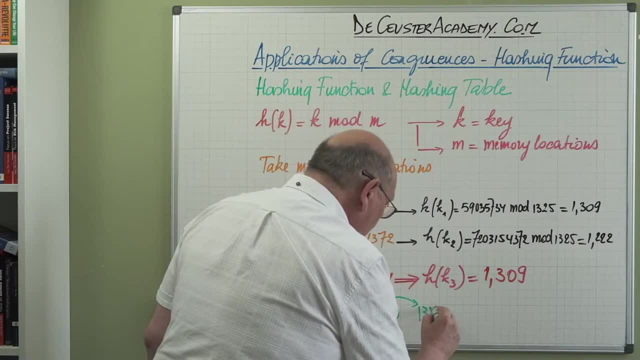 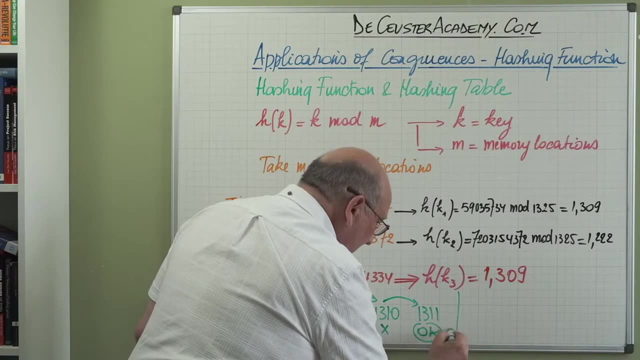 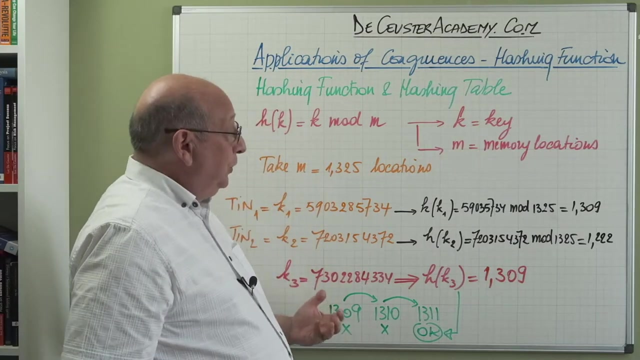 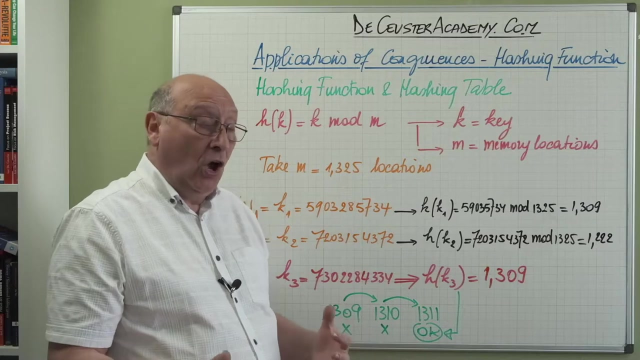 continue. then we go to 3,000, 1,311, and here we see it's free. so k3 is stored in memory space 1,311. now this is what we call a collision, and the collision is when we have a memory allocation of an input that is already used, the memory. 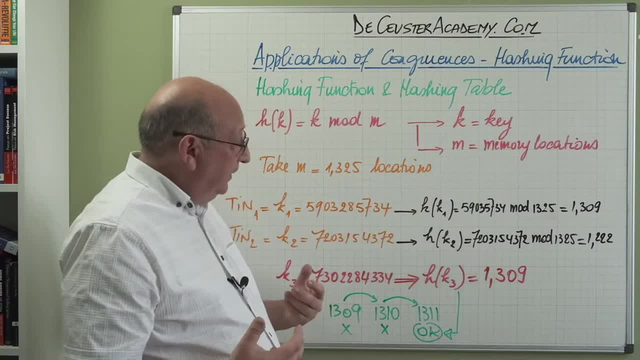 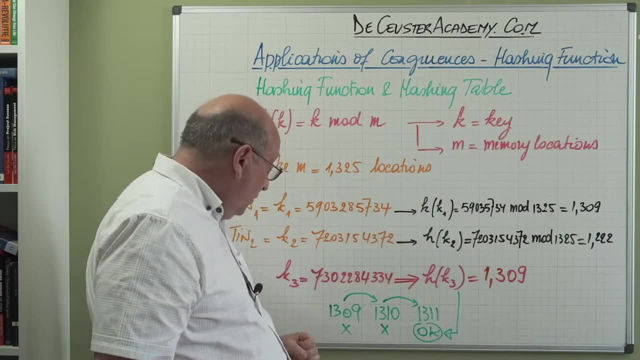 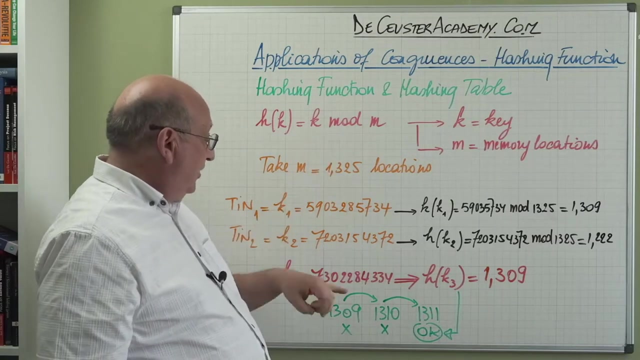 space is already used. now this can happen and of course, it's not nice to have it. it will lead to more calculations because we have to find the next spelt, and so on. now we can do that in a different way. we can say that it's one spot, we add one spot, or we can jump. 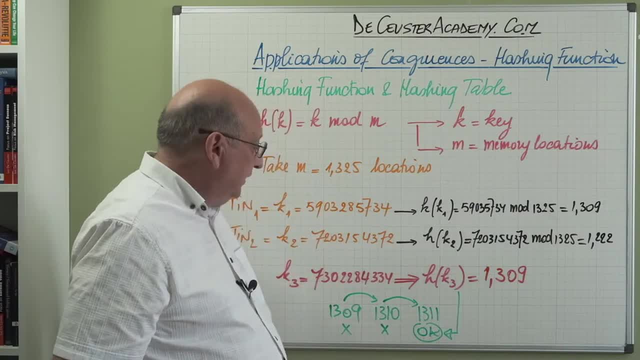 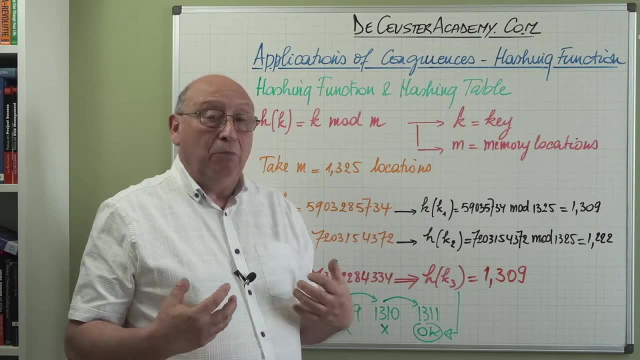 to three spots and things like that. so there are different possibilities. now, how can we avoid collisions? now it's clear that collisions will occur when we have a collision and when we have a collision, and when we have a collision and we will wait to have so for, for example, we had an analysis. we 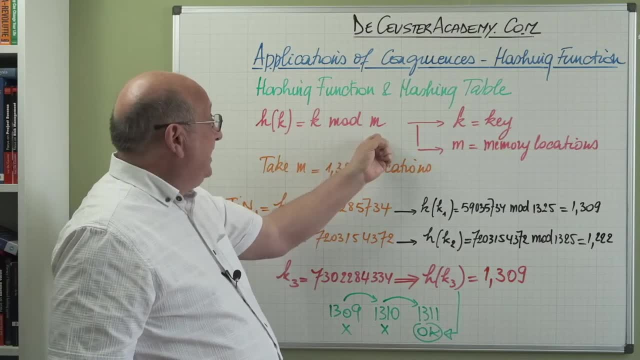 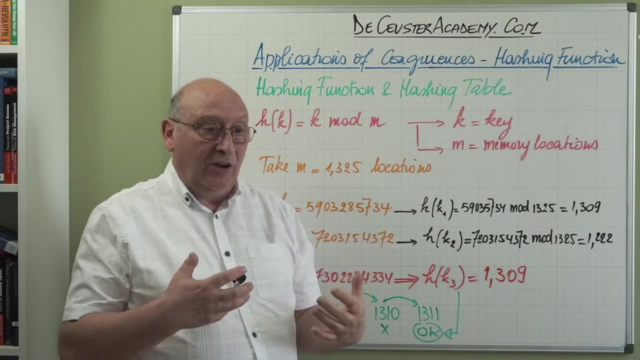 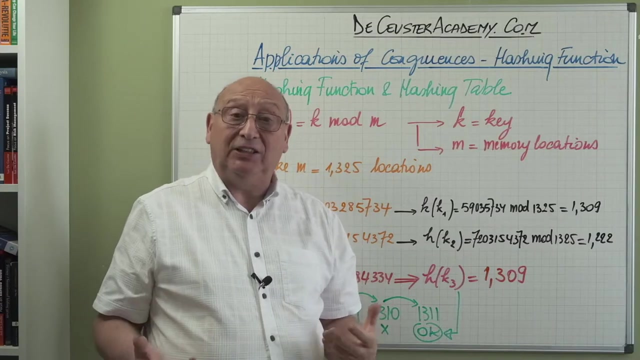 wanted toiz benut it in our data. then we need an analysis of what if a enrolled person called: this is the pivot- again interesting because it's very significant and we can strowane type. that usually isn't. that's it still published? it is correct, it's still. it's there for me. but let's to another. 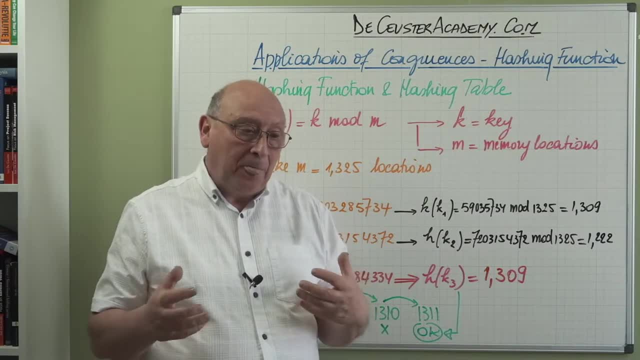 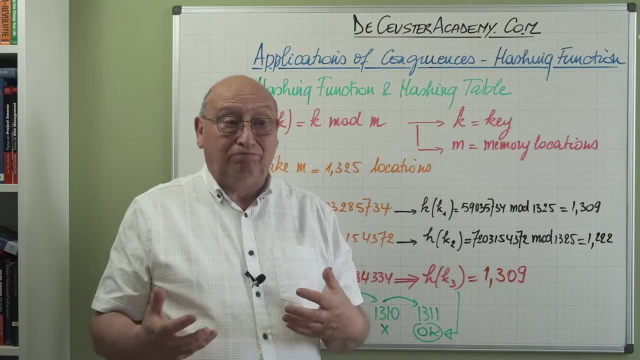 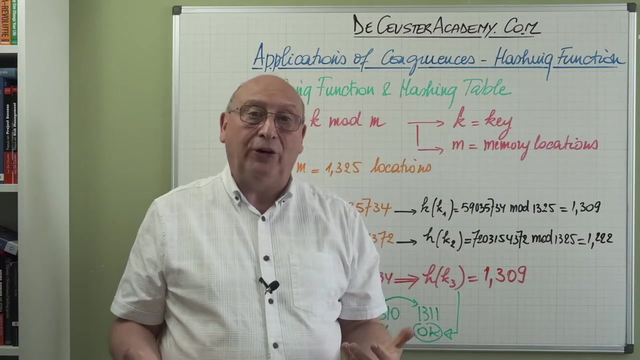 빔bon. I speak about mobilization of memory spaces. OK, now we have an analysis of the possible Buttons, So can we do estimated the number of sum we consider and wishes expecting to enter into the system, we can allocate a larger amount of memory to store them. 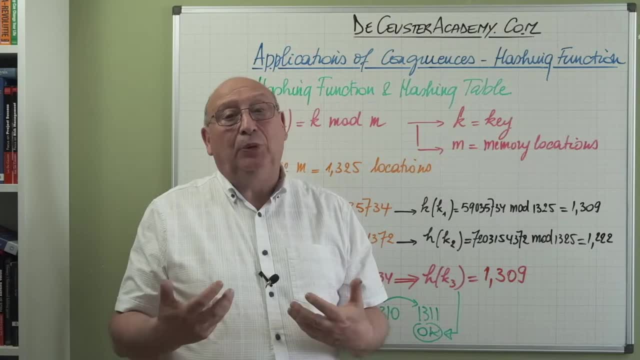 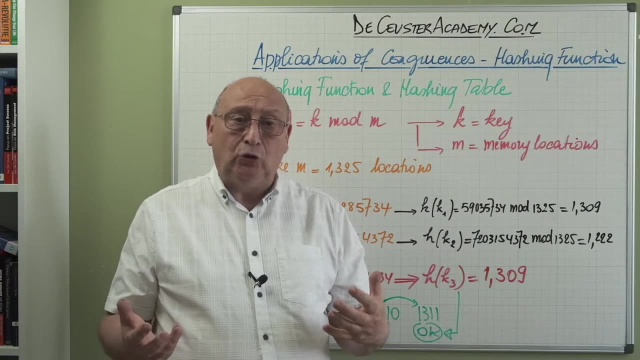 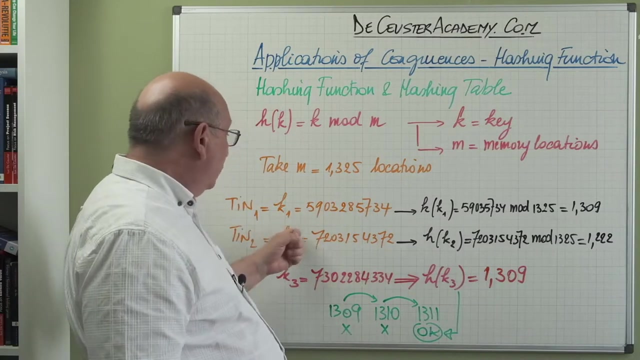 It will avoid the collisions and it will reduce the calculation time. Now, why is it also important to avoid collisions? Just imagine that you want to do the inverse function. You want to find the data. So, basically, what you're going to do is you're going to calculate the key again. 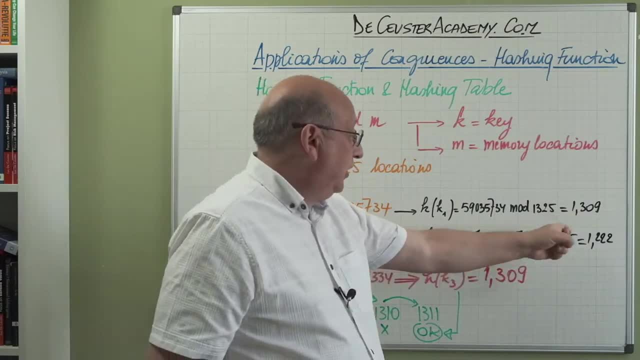 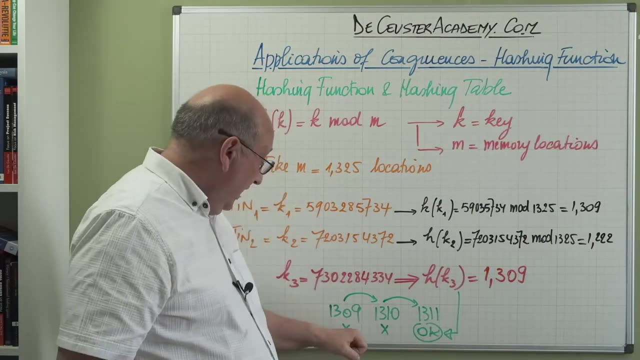 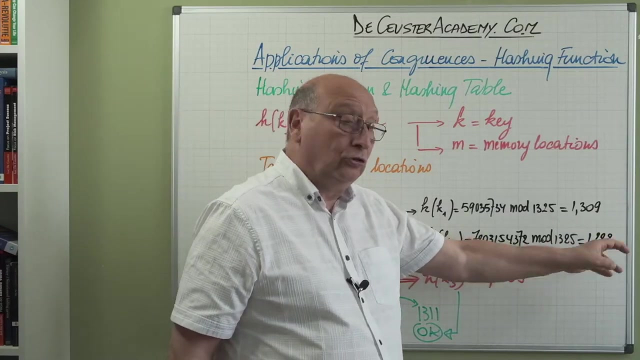 So you find for K1, 1,309.. You go to the position. You say, okay, we found the value. This value is K1.. So it is confirmed. The same for K2.. You will go straight to 1,222.. 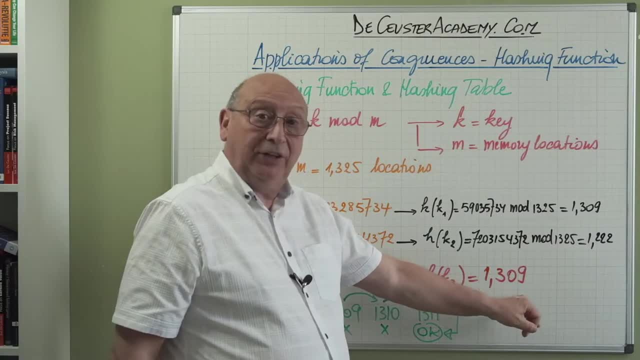 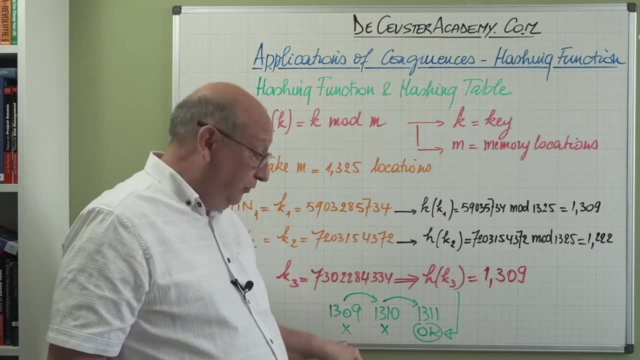 It's not a problem. But what happens with 1,309? With K3?? K3 will have a look here due to the hash function. K3 will have a look here. due to the hash function, We find it's 1,309.. But we see that this value is not equal to K3.. 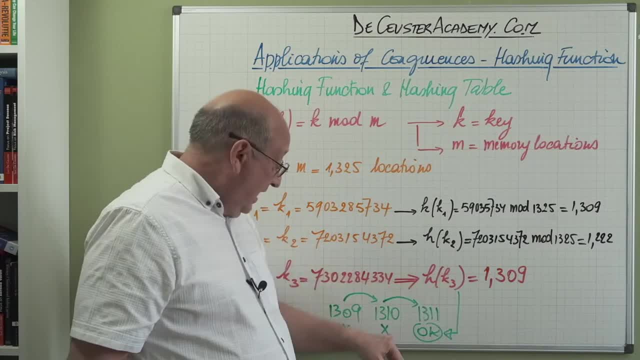 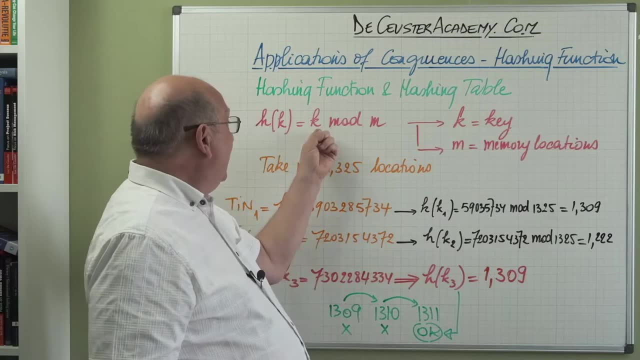 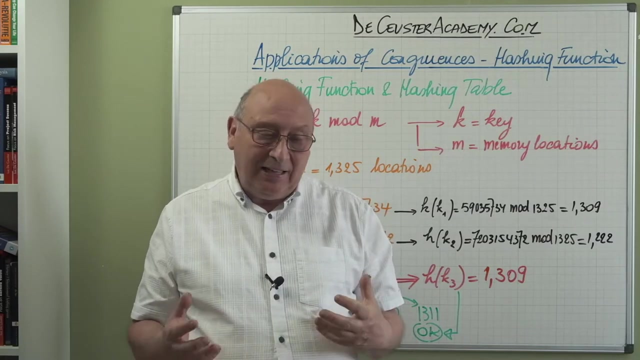 Then we go to the next one. It's not equal to K3.. And again to the next one until we find the value that corresponds. Now you can imagine when K and M are very close that M is only a little bit larger than K. We will have more collisions And first of all, 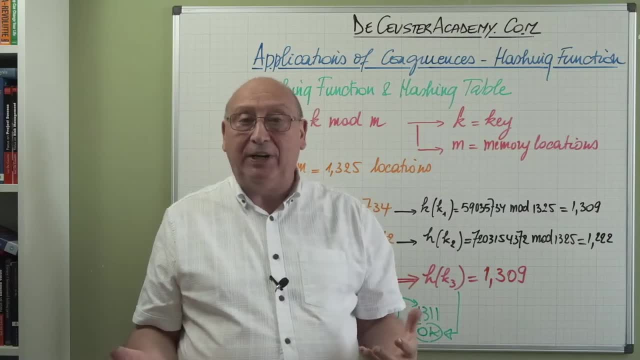 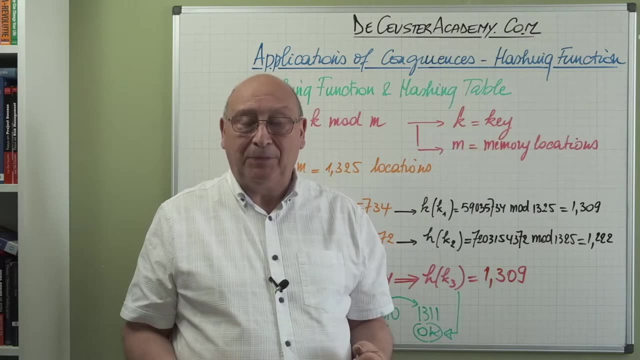 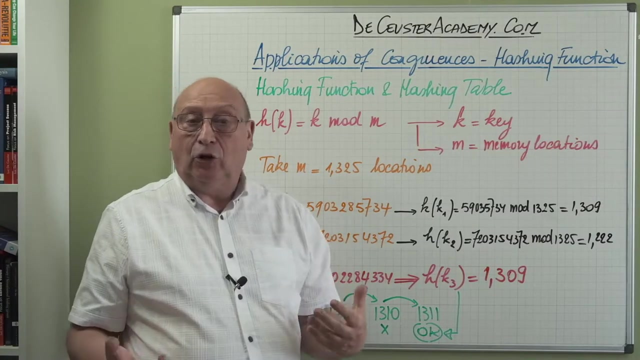 the time to store a number, Some numbers somewhere in memory will increase, But on the other hand, we will have the same problem when we want to retrieve that value. Now, we've been looking at this. We looked at this number. Now there are different ways to deal with those numbers. Let's have a look. 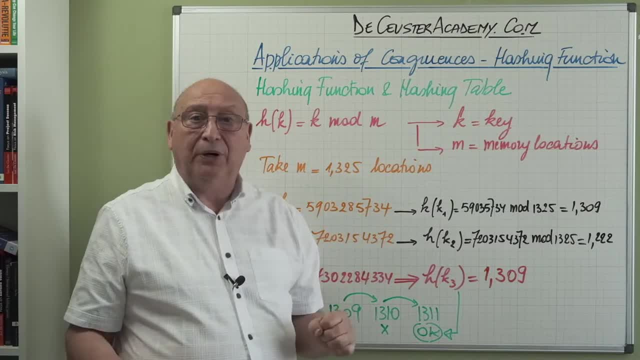 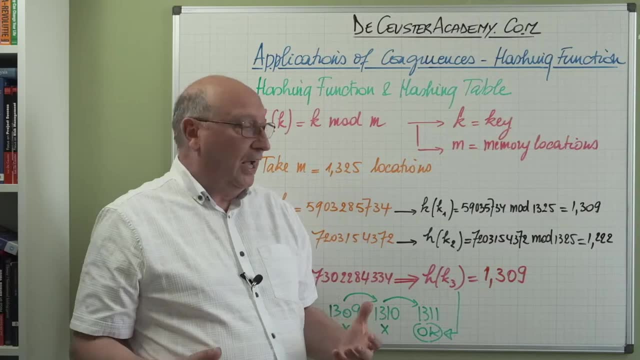 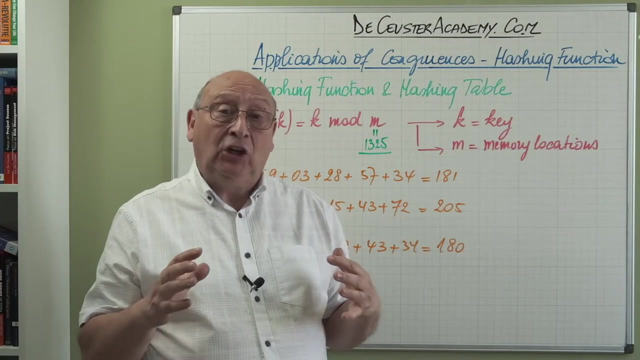 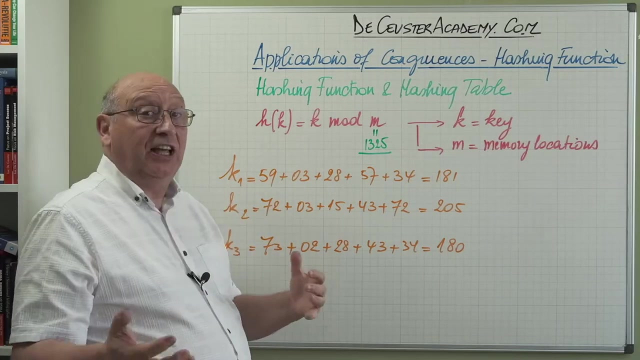 at a different way how to use these numbers and show you how this alternative can also be used to calculate the memory position. Another way to deal with the hash function is, in fact, to get the numbers written in a different way, So we still have the tax identification numbers or the personal numbers. 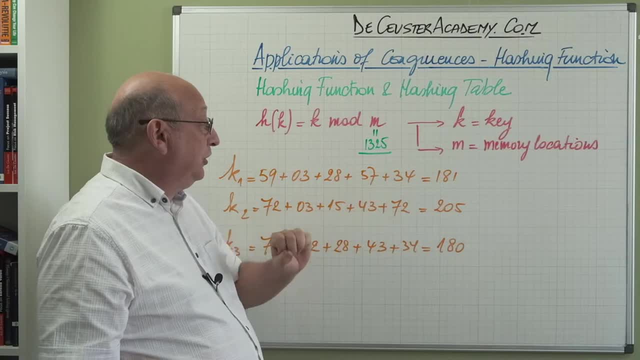 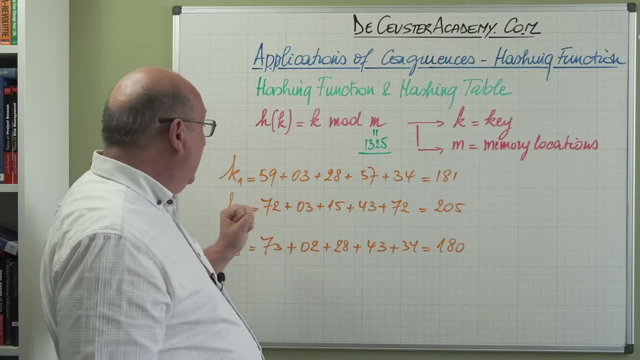 which are 59,, 03, 28,, 57,, 34.. But what we're going to do is we're going to just add those numbers. So basically, we maximally have 1,, 2, 3, 4, 5. The maximum number we're going. 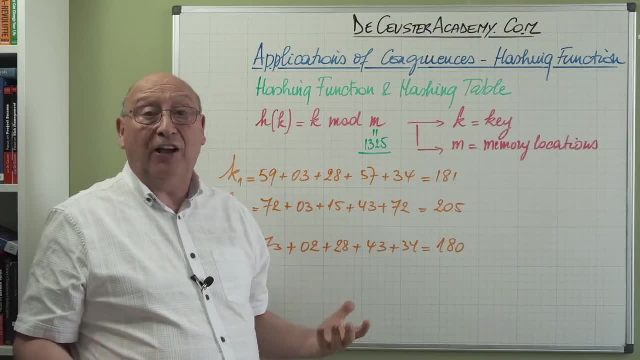 to have is 1,, 2,, 3,, 4, 5.. The maximum number we're going to have is 1,, 2,, 3,, 4, 5.. The maximum would be around 500, a little bit less than 500.. Now, basically what we have. 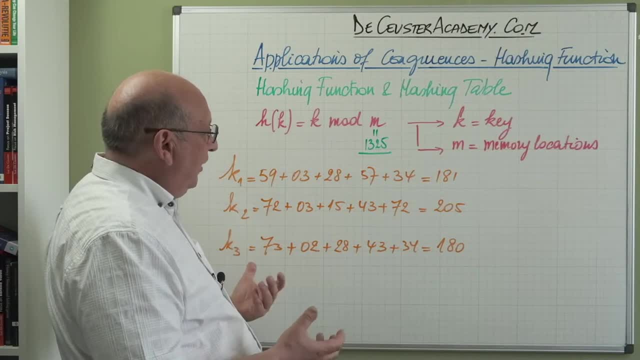 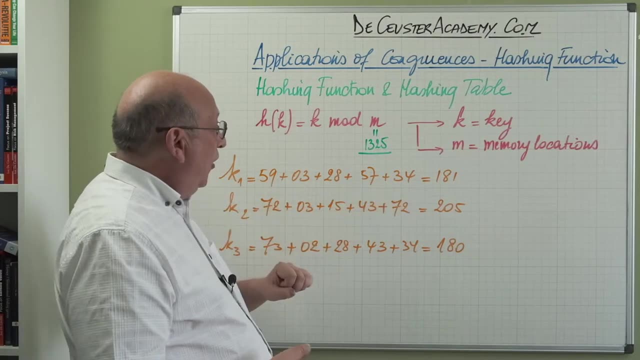 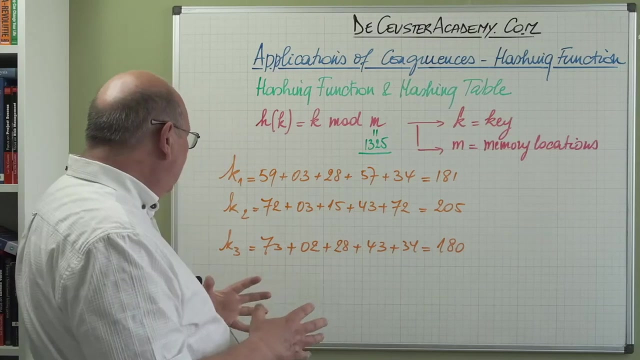 here in those numbers, is that we can find a different allocation. Now we will see. with those numbers, since we have a maximum of 500 and we have more numbers, we may have more collisions. But this is something else that we will look into later When we look. 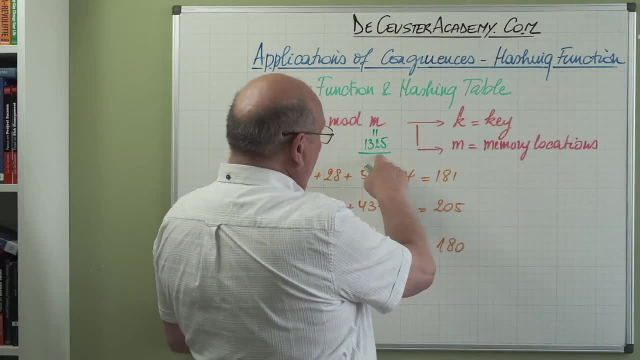 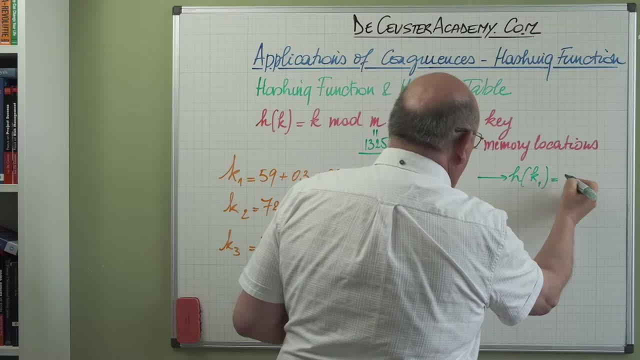 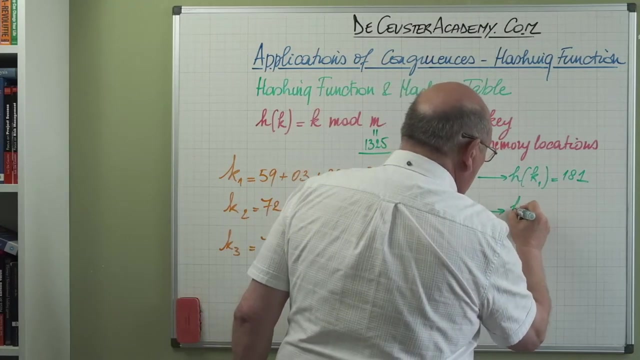 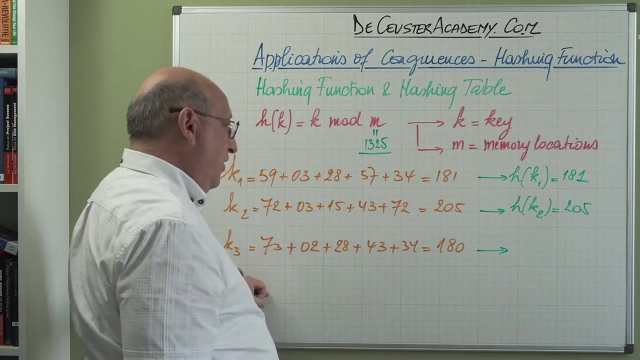 at the numbers here. So here at 181,, modulus is 1,325, so h of k1 is equal to 181.. The same thing for k2, this is 205, and the value for k3, h of k3 is equal to 181.. And you can see here this: 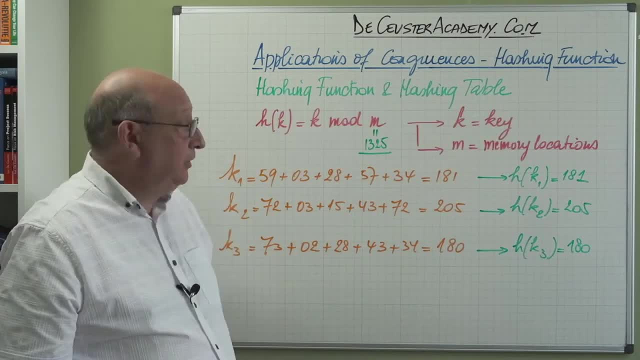 is vice versa. So we could see the difference between these numbers that I have within those numbers. But again, we can also do earlier this one to get the Ungugnzi equations, And Now here we have those numbers. it may not be the best way to deal with it, but 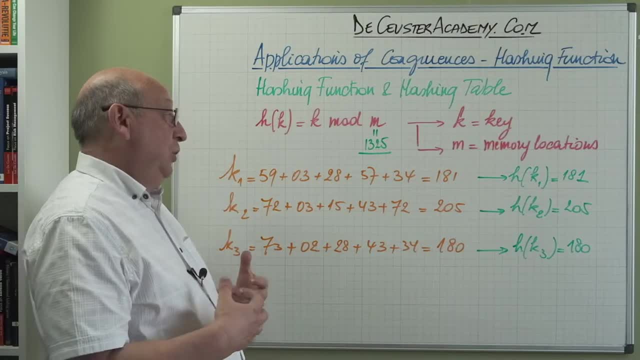 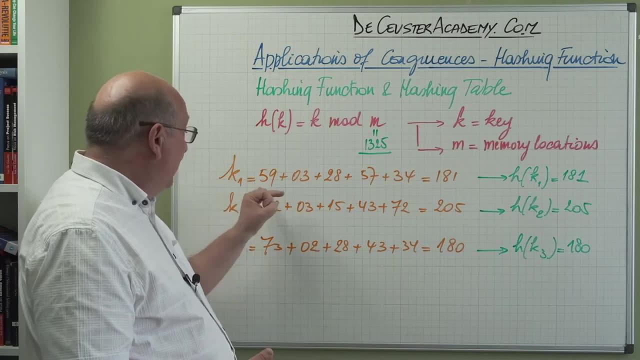 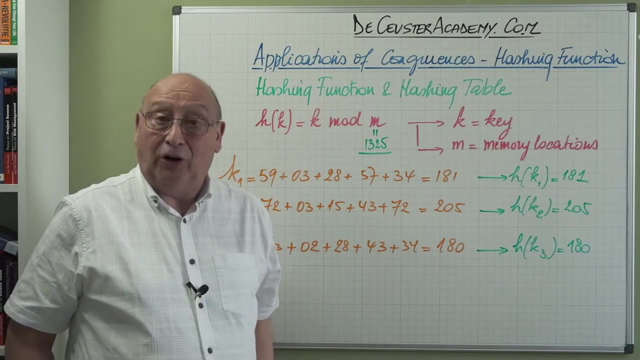 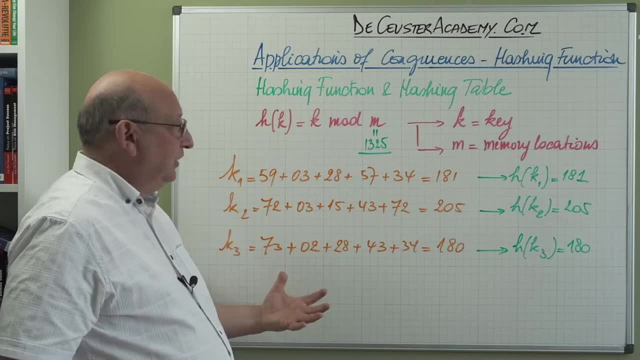 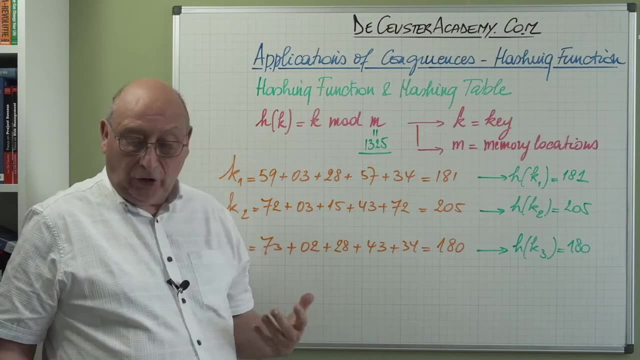 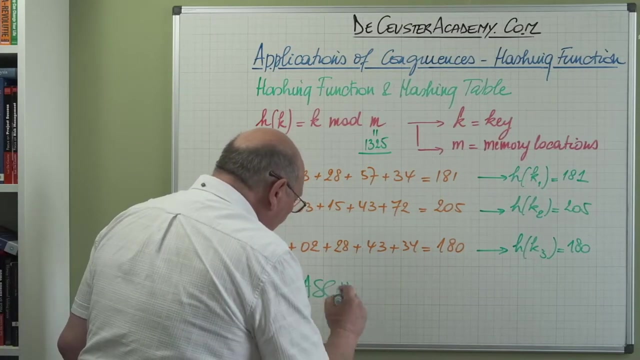 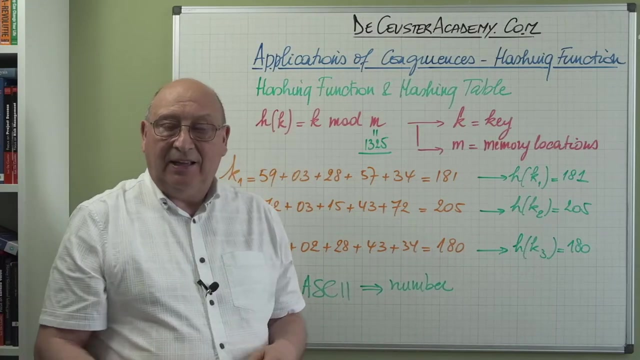 did. I want to show this. Well, we have different elements that we can consider And when we are looking at using letters or other symbols, and what happens in computers, there is the ASCII format, which gives a number for every character, every letter, every number that you 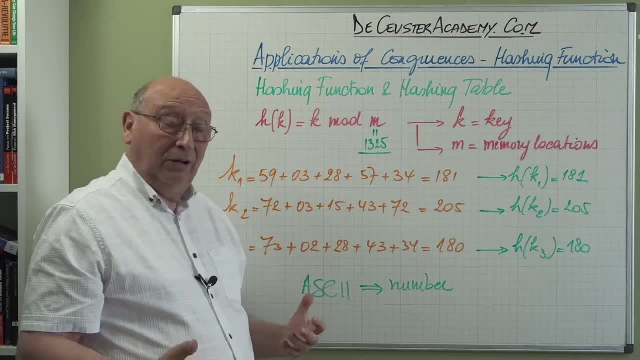 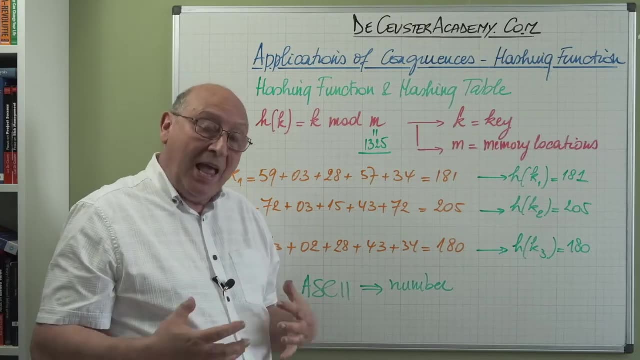 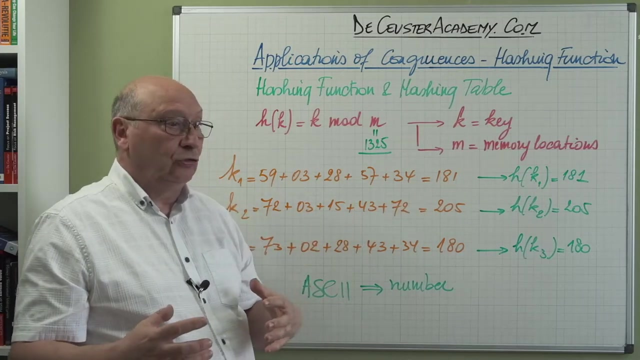 have. every symbol, a dollar sign, a space, a point- has a specific ASCII number, And what we're going to do? instead of sorting numbers, we're going to translate those strings. for example, my name Luke. we're going to translate it in a set of. 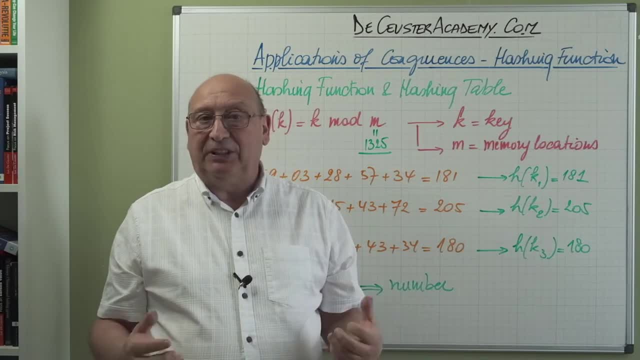 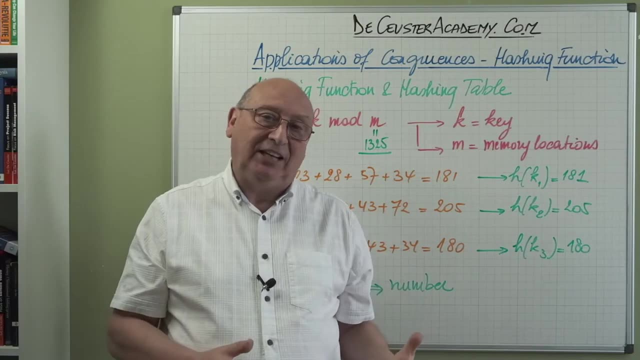 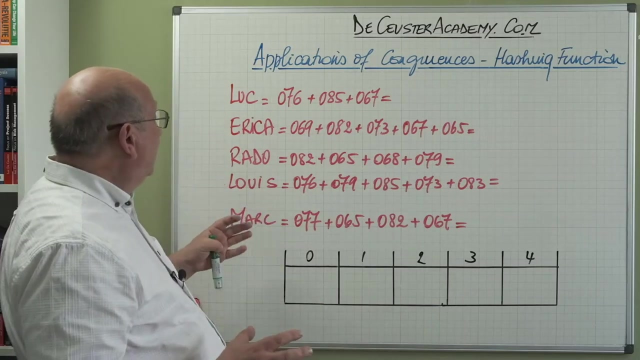 ASCII numbers. Typically, they are represented by three numbers. Let's have a look. Let's have a look how this can work and how we can put this in a hashing table. Here we're going to use the hashing method to allocate memory spaces to. 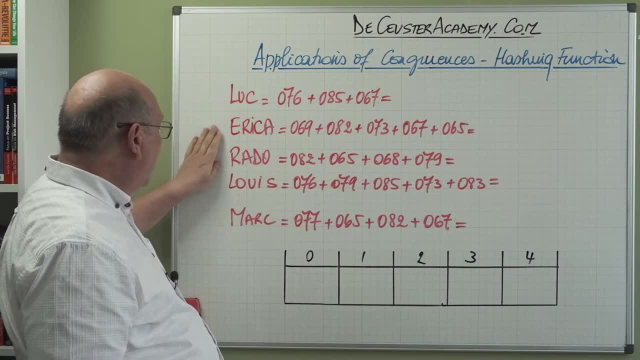 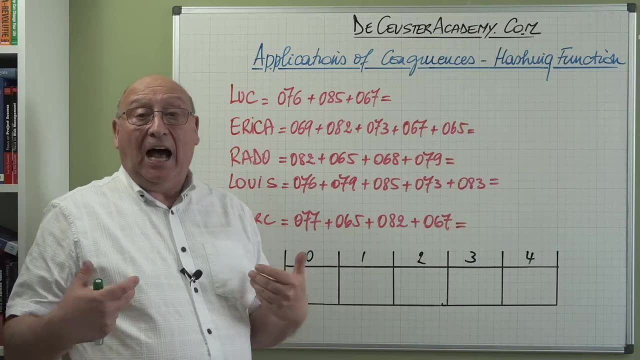 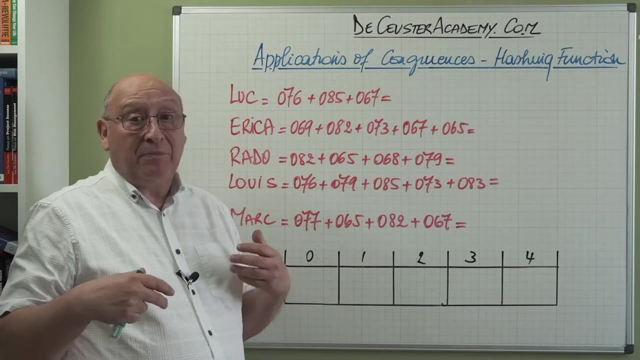 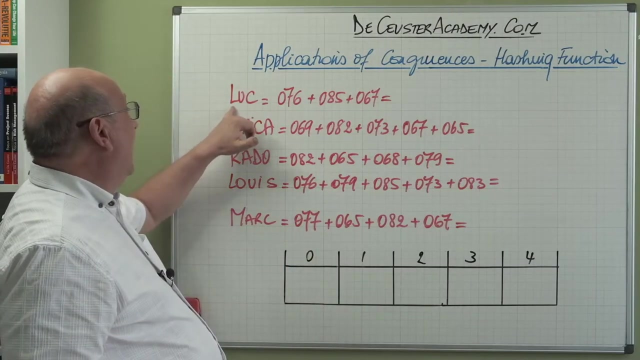 different people: Luke, Erika, Rado, Louis and Marc, or Mar like the French would say it. Now, first of all, we have to identify the different ASCII codes of the letters. Be careful: there is a different between, let's say, the small and the capital letters, So capital L and small L. 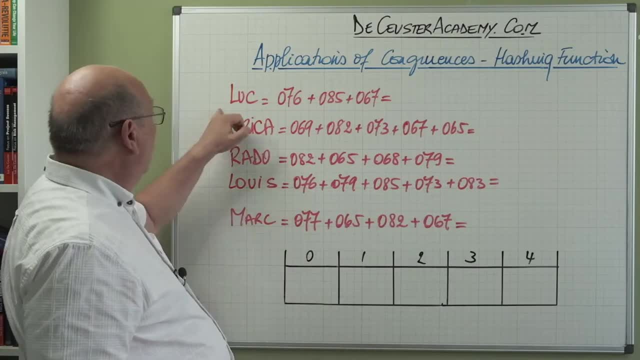 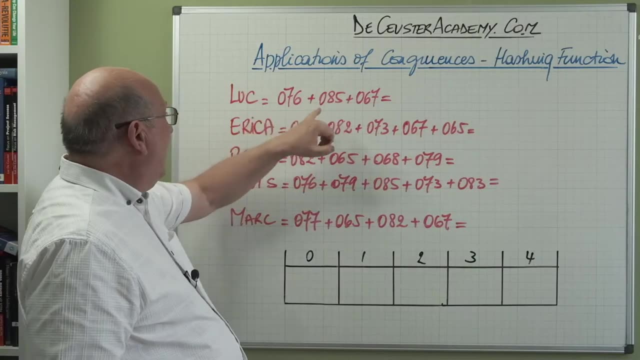 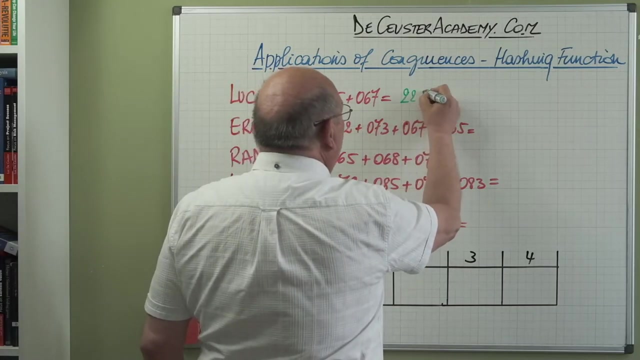 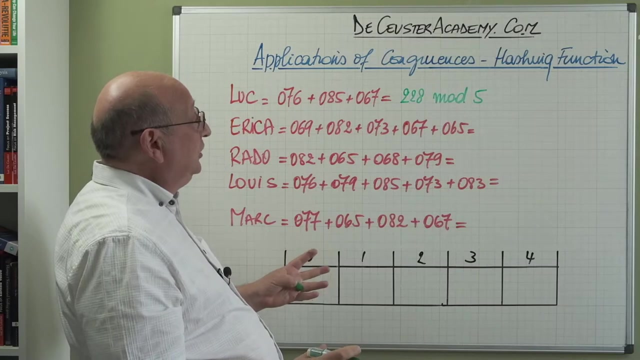 have a different ASCII code. So for Luke this is 076.. I considered all capital letters. For you it's 085, and for C it's 067.. When we add all of them we find 228 modules. We have to add 5 because we have five memory spaces. So we consider here: 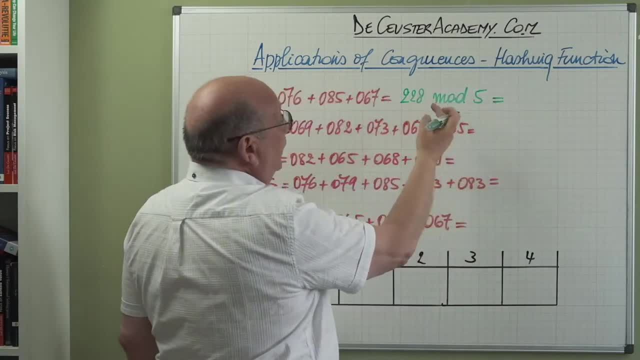 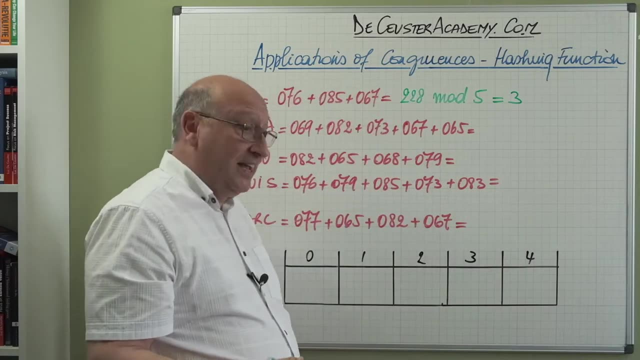 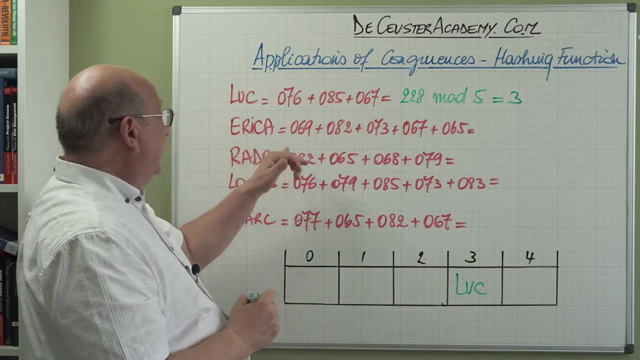 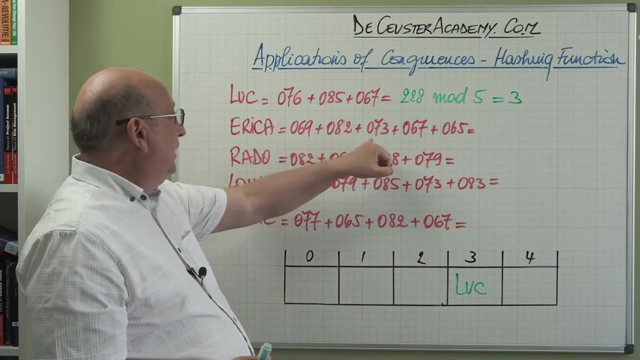 modulus 5, which in this case 225 is, let's say, divisible by 5.. So I have a remainder of 3.. So basically, I will put Luke in space 3.. Now the next one, Erika. still okay, we're just starting with it. So E is 069, R is 082, I is 073, C is 067. 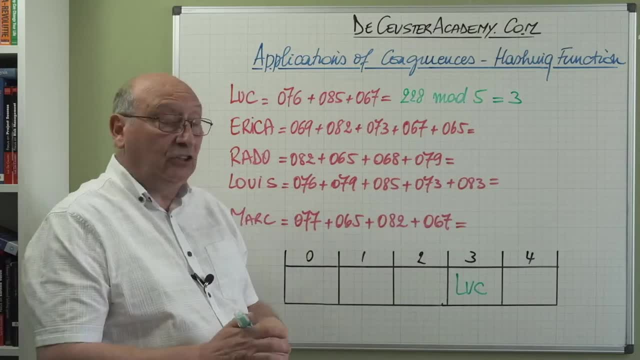 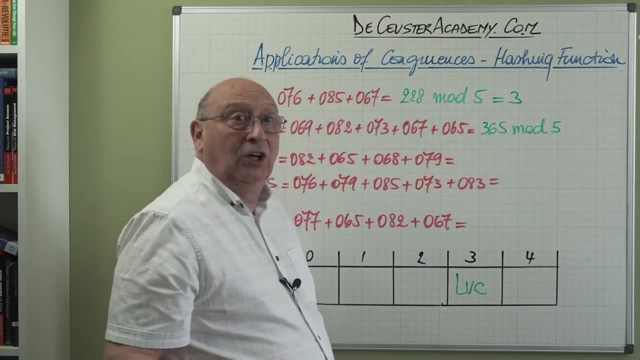 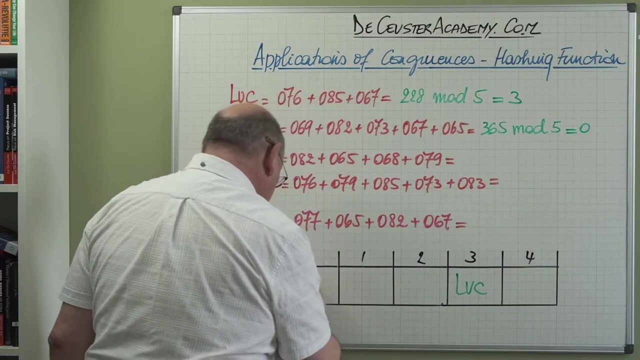 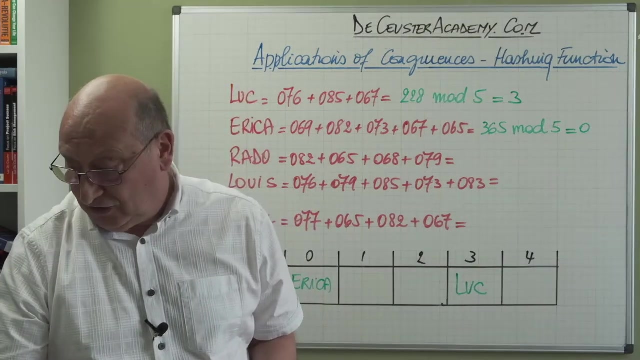 and A is 065, which gives us a total of 365.. Modulus 5,, which gives us equal to 0. So we put Erika here. So when we have Erika in this spot, we find immediately that. oh, sorry, I made. 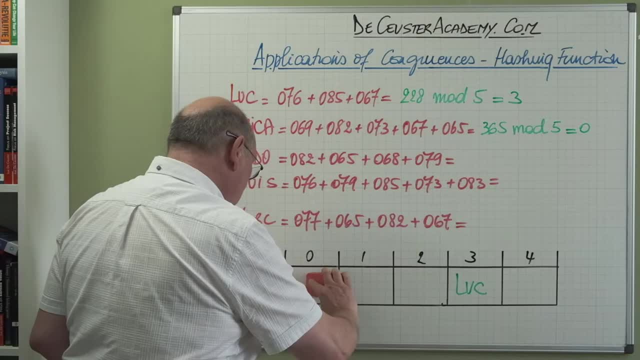 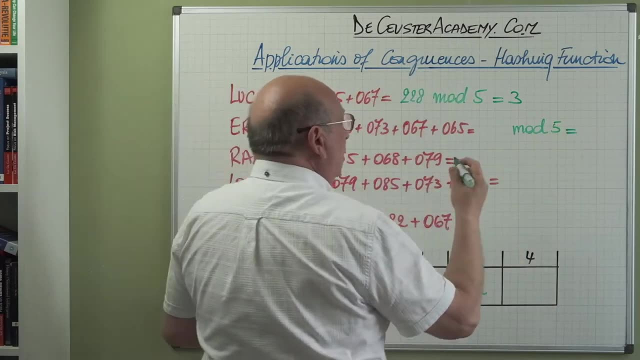 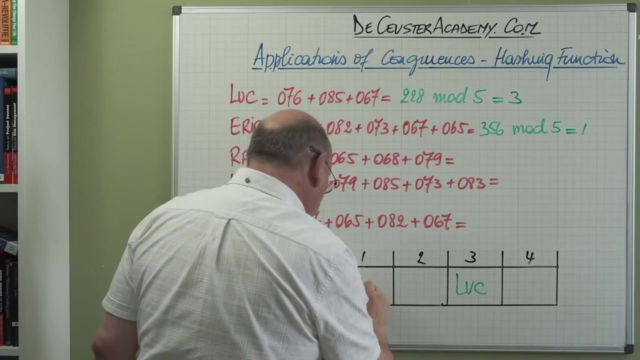 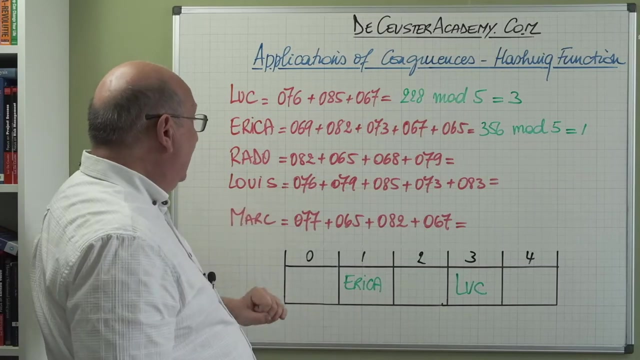 an error here. This is not 65, it's 56. Sorry for that, So 356, and we find modulus 1.. So we put Erika in memory space 1.. Okay, we continue with RADO When we take the sum. these are the ASCII codes. 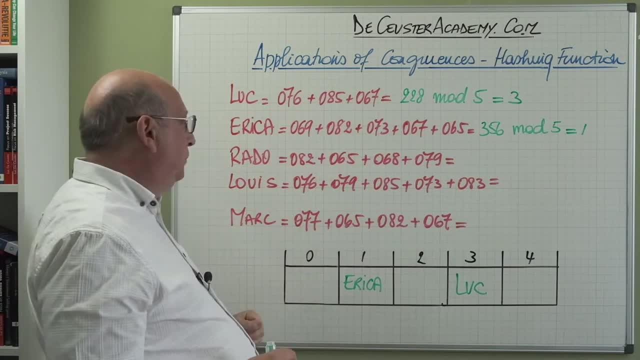 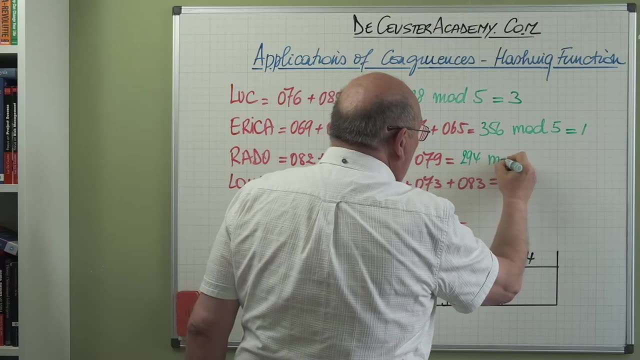 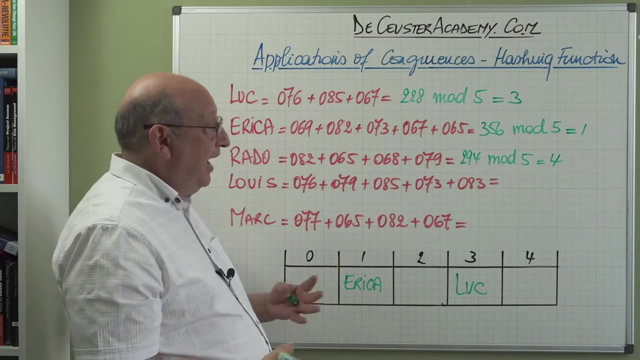 You can find them on Google. They're fixed for all computers so that we can use it everywhere. And we find it's 294 modulus 5, which gives us 4. We have: 290 is a multiple of 5, so 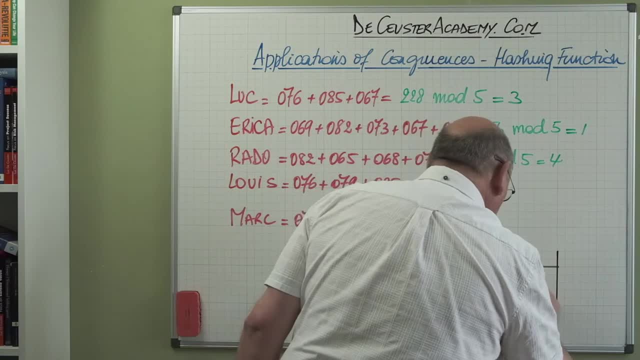 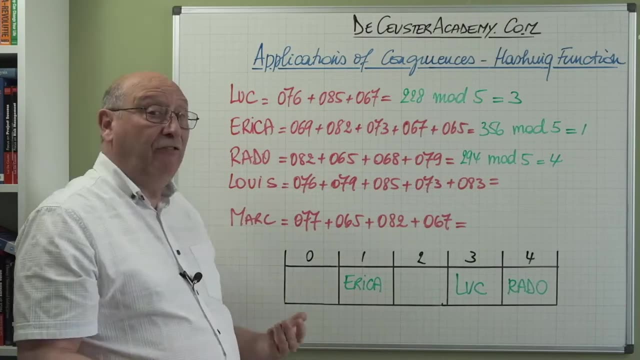 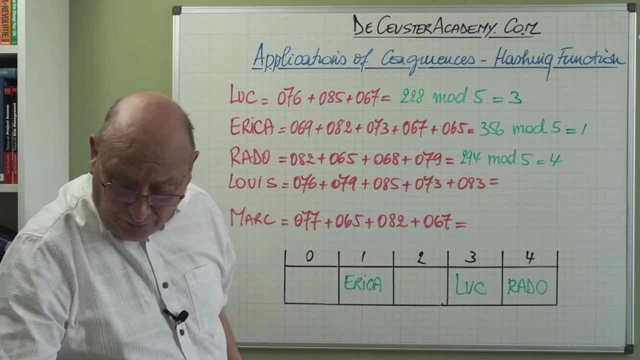 4 is the remainder And we find RADO 0. Here Now we have 5 numbers, 5 names, so we will have 5 spaces. It means we can expect some collision. in this case, When we look at Louie- and I will take a different color to show it- I find when I add all of 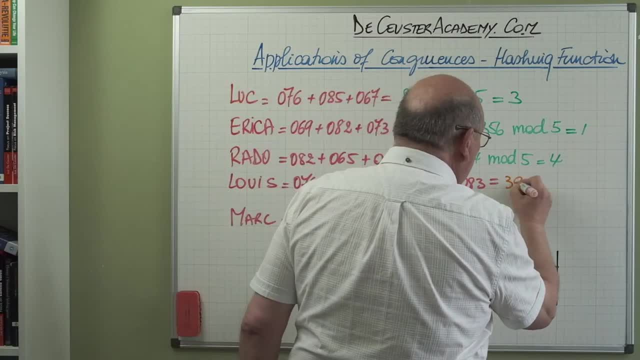 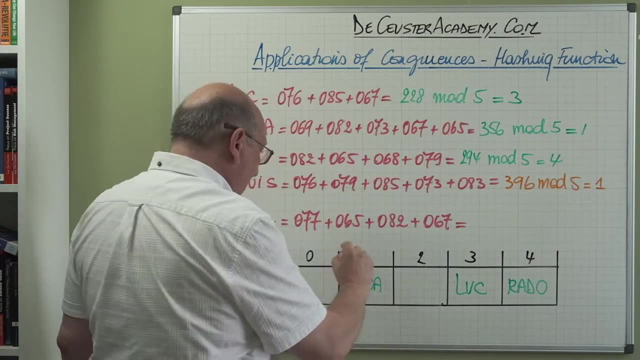 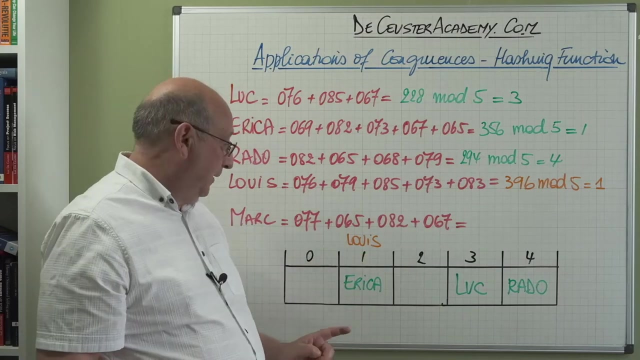 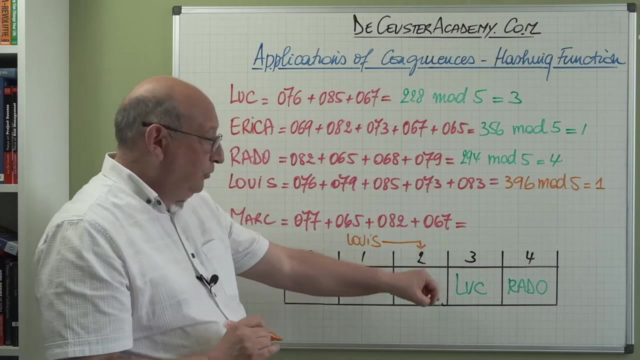 those. I find 396 modulus 5 is equal to 1.. So basically, I want to put Louie Here, But Erika is already there. So what we're going to do is to move to the next space And we see 2 is free. 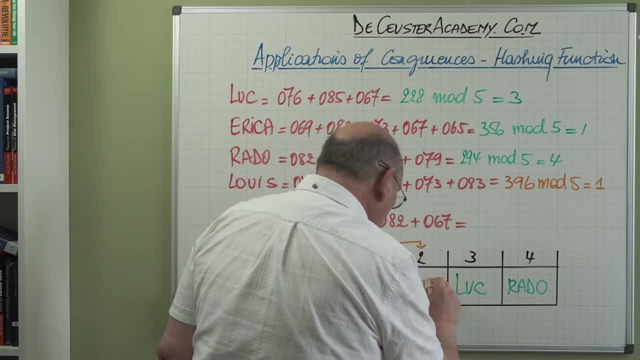 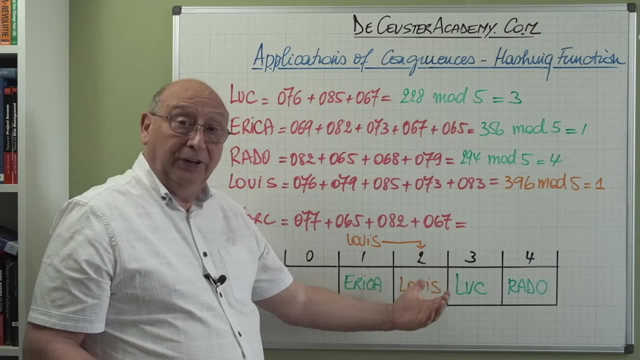 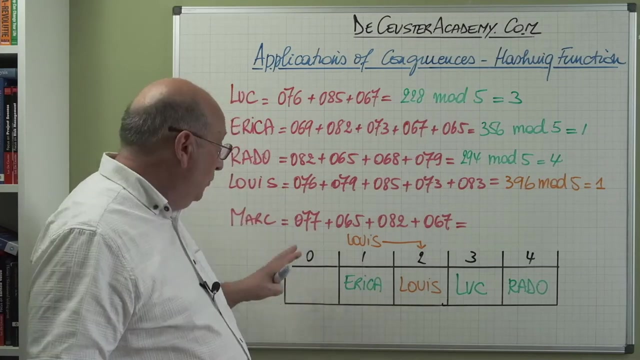 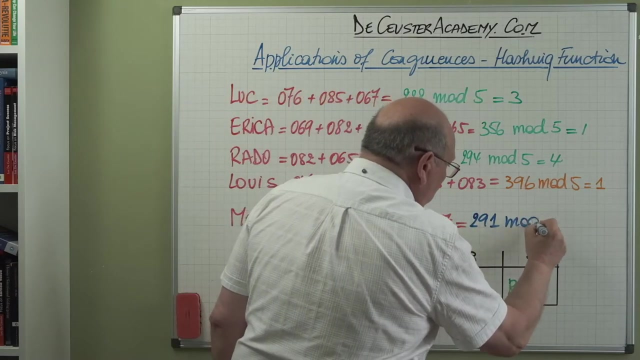 So I put Louie in space 2.. So we have a collision, but we solved it by moving Louie to the next space. The last name to deal with is Mark Or Mar, Like the French would say. And when we count here all these numbers together, I find 291 modulus 5, which is equal to 1.. 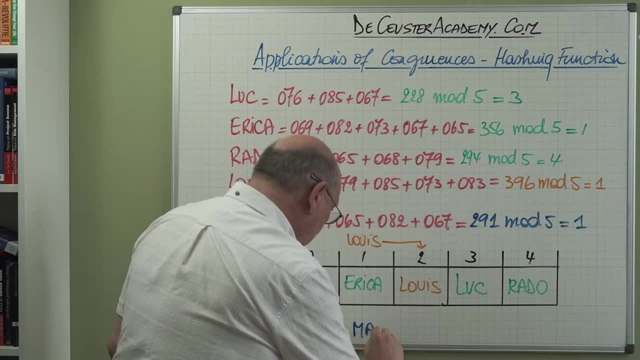 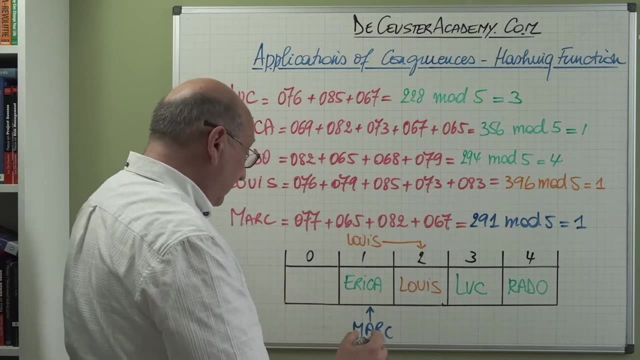 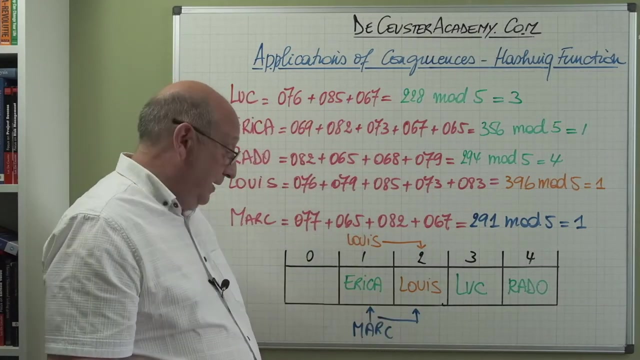 So basically, I want to put Mark here, But I see this is not free because Erika is already there. So I go to the next step And I see that here is Louie. I go to the next one to 3.. 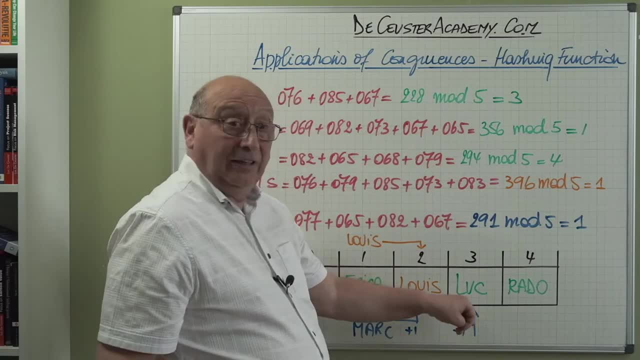 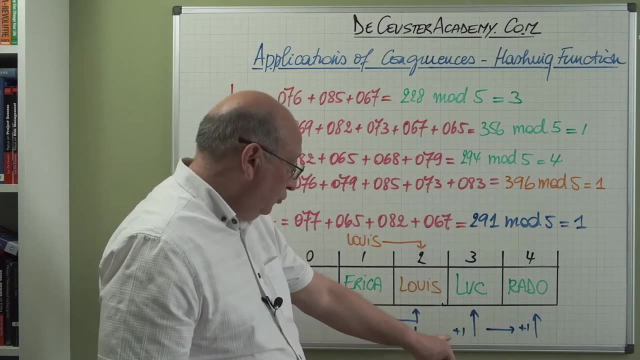 So plus 1, plus 1.. I find Louie is in this spot. I go to 1 again plus 1.. So I added 1, 2,, 3, 2, 1.. I come to location 4.. 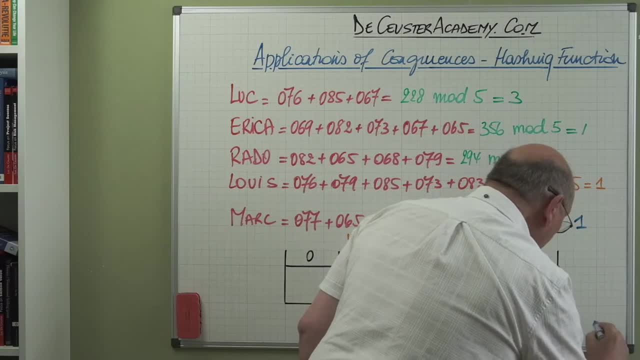 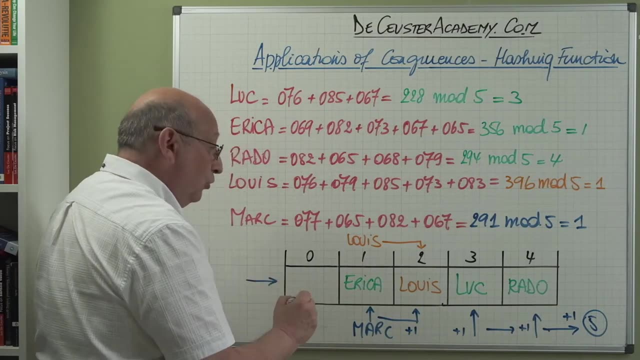 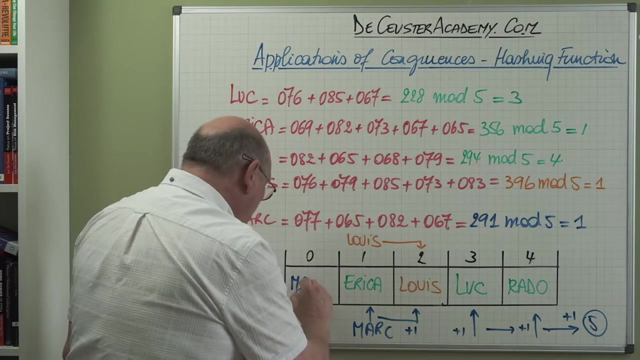 And I add plus 1, because it's still full. So I have 5.. But 5 modulus 5 is 0. 0. 0. 0.. So you can see that now, in the same idea, the ambition is to put Mark into the hashing. 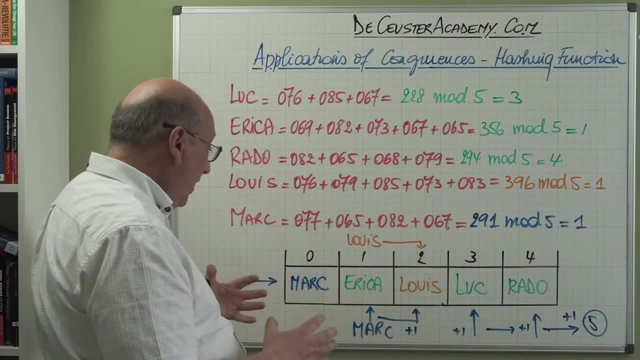 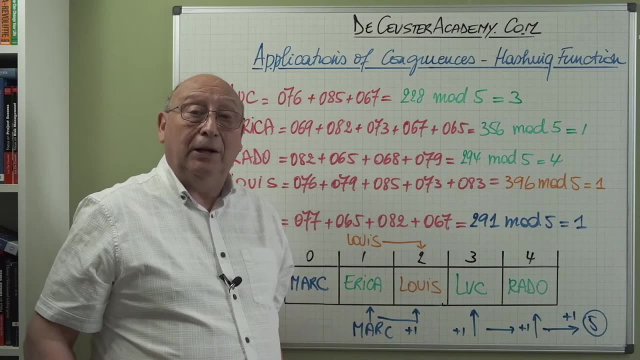 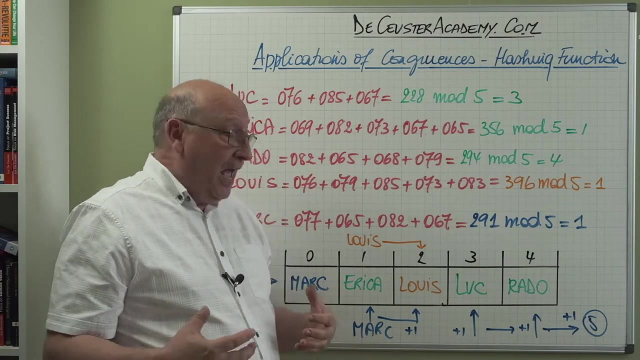 table is to put Mark in position 0.. So we see here how it works And we have five data, five names, to put in a memory composed of five memory spaces. It is clear that we expect collisions Size and that's all. 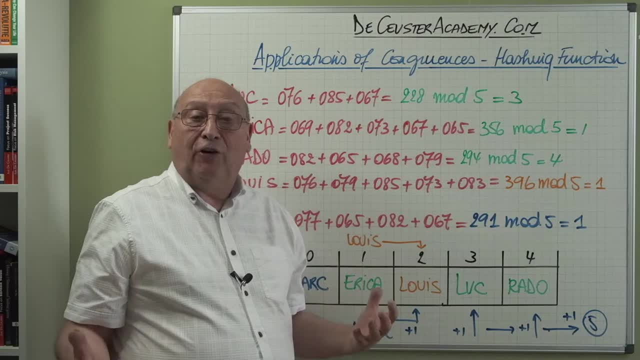 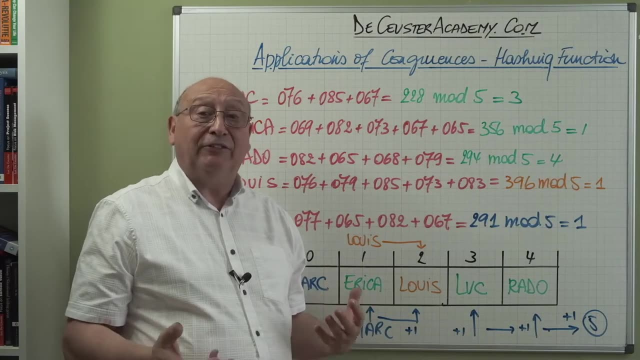 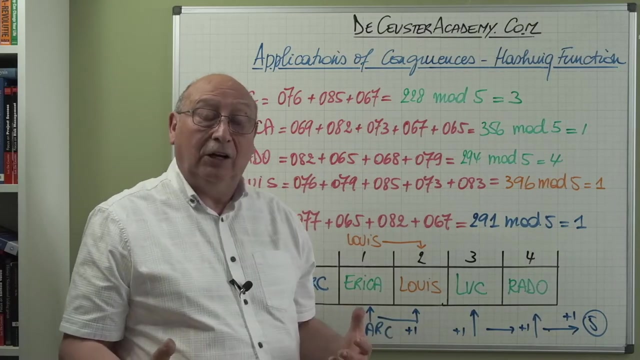 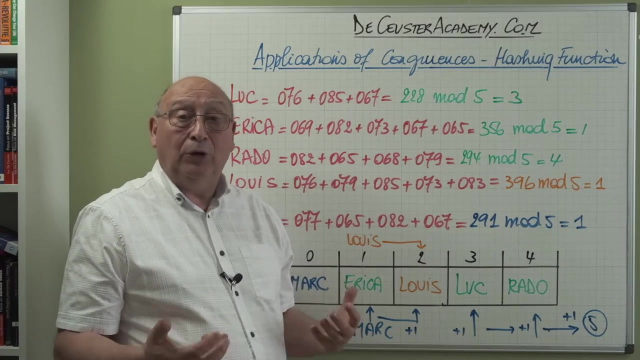 2.3. footage: 100 names and we put, for example, 500 memory positions. of course those positions are fixed, but we will not have so many collisions, which means we don't lose so much time by resolving collisions and we reduce the time to find the data when we know the key and the memory space that's connected to. 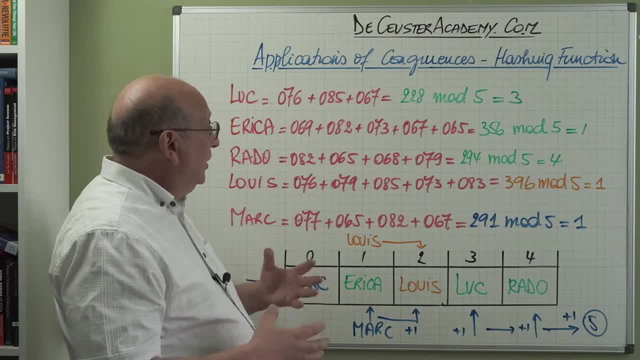 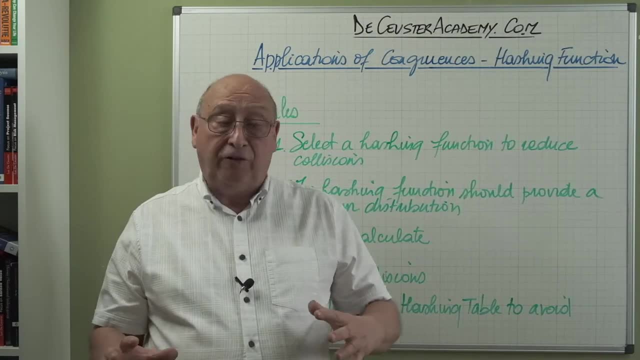 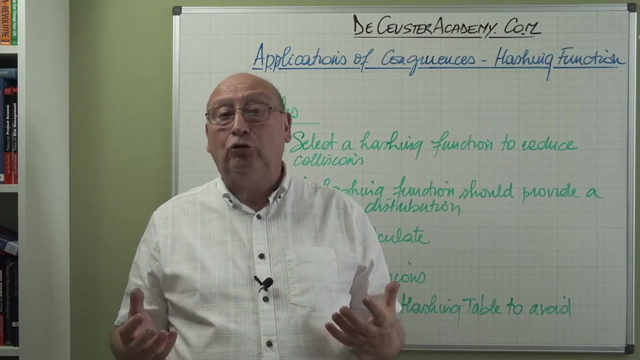 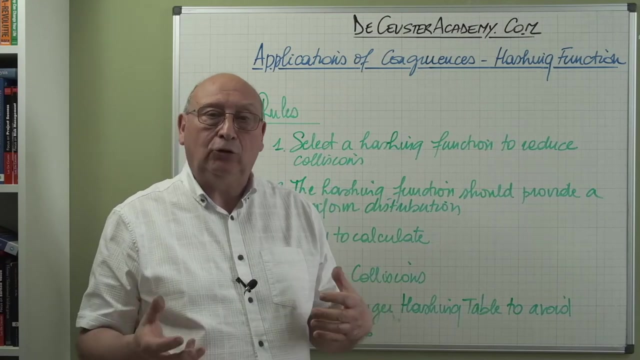 it. so that's one exercise. let's have some look at some other things related to the hashing table. we saw the principle of creation of the hashing table, how to use the hashing function and how to resolve collisions. now, when we look back, we can formulate some rules that we have to take into account when 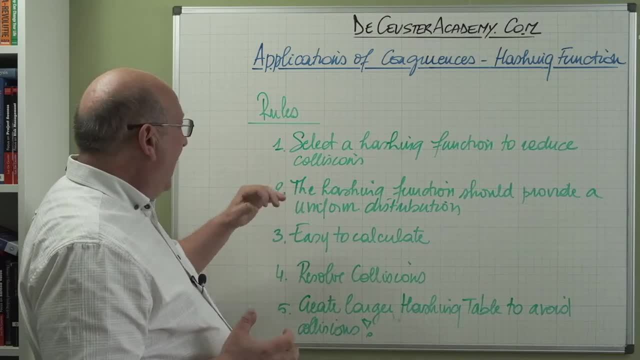 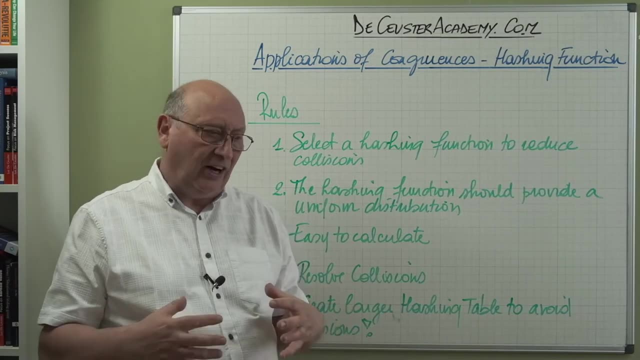 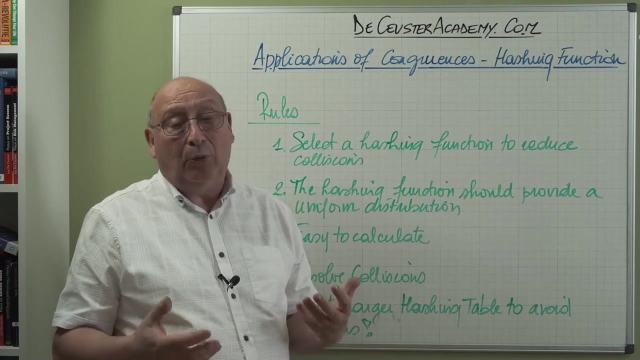 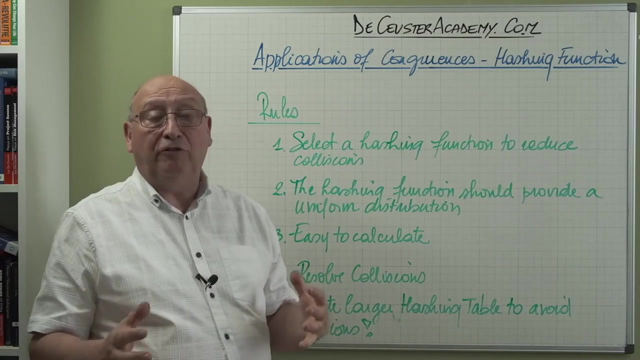 we create a hashing function, first we have to select a hashing function that will give us the least possible collisions. there are different hashing functions that you can find and you have to understand what data you have and what hashing function will be ideal for you. the hashing function should provide a uniform distribution. it means that the 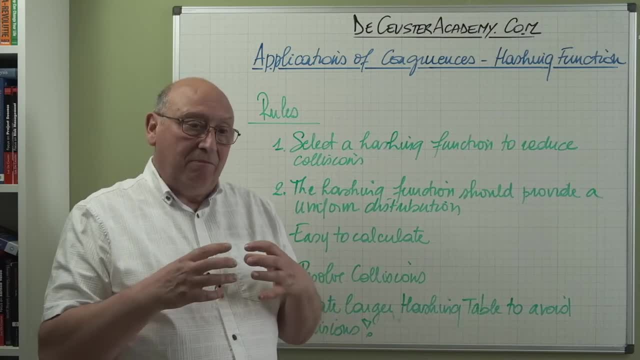 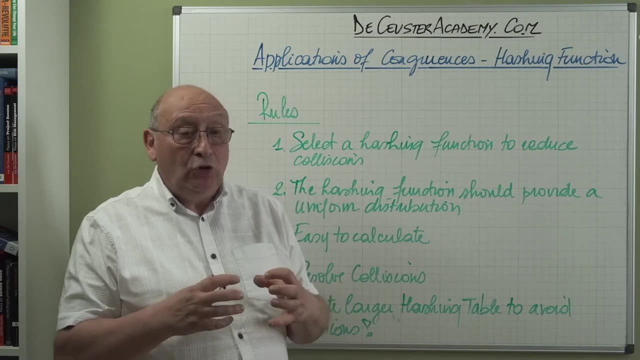 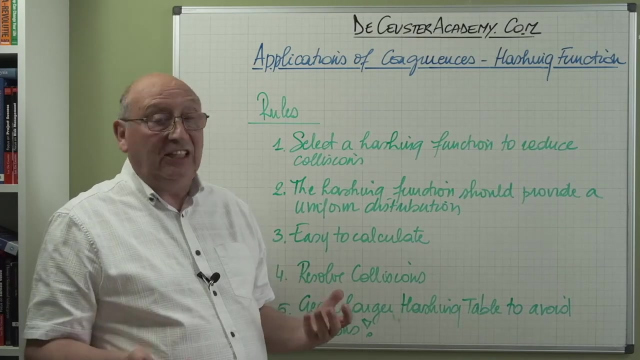 numbers that come out that every memory space has a different number of collisions. it has the same probability to be selected. so that's very important because then you will have no collisions, or a minimum of collisions has to be easy to calculate. easy functions are easier to calculate. take less time, take less. 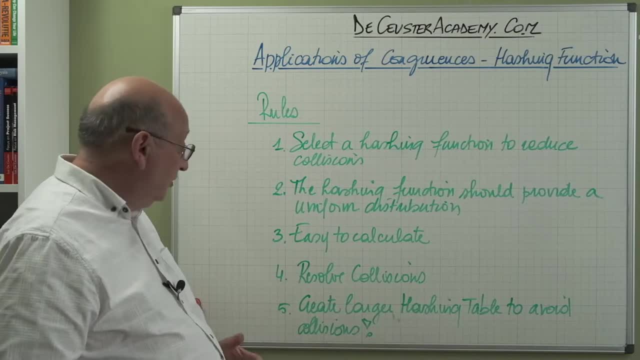 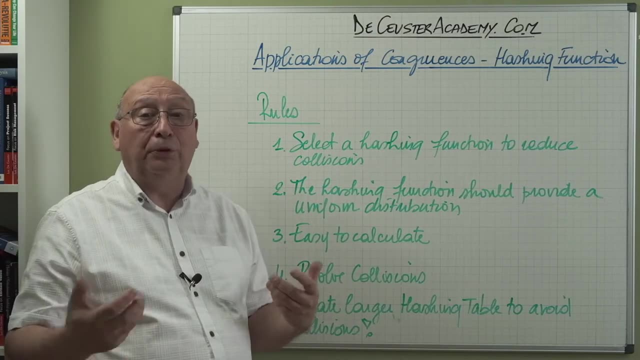 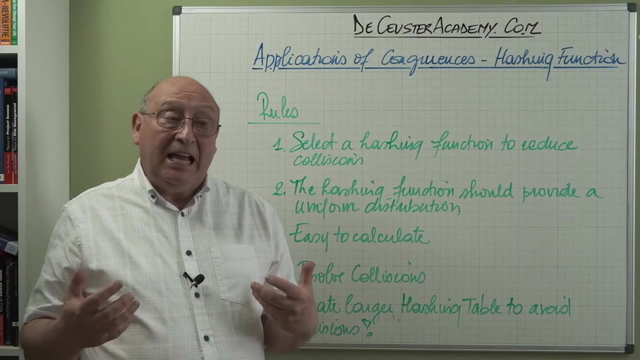 memory, memory. so it's an advantage it's not so complicated. we have to find a way to resolve collisions. how will we do that? we will. will we jump one position, two position, three positions? it depends on what we want to do. and a last thing: what is important is that we have to 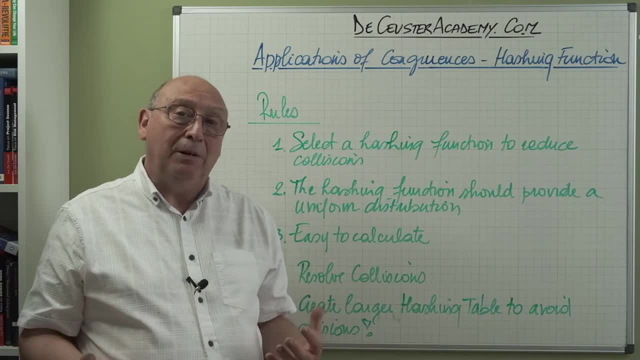 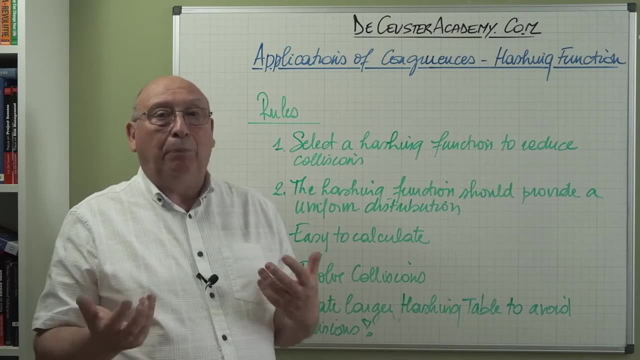 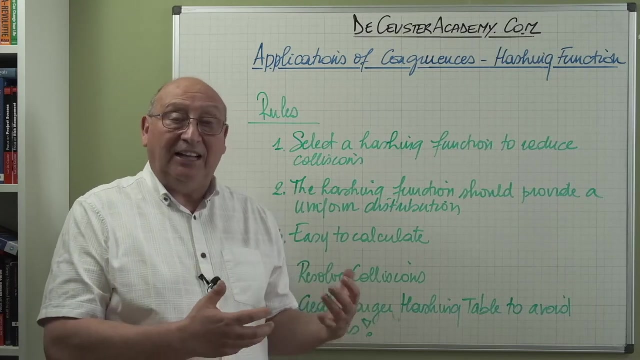 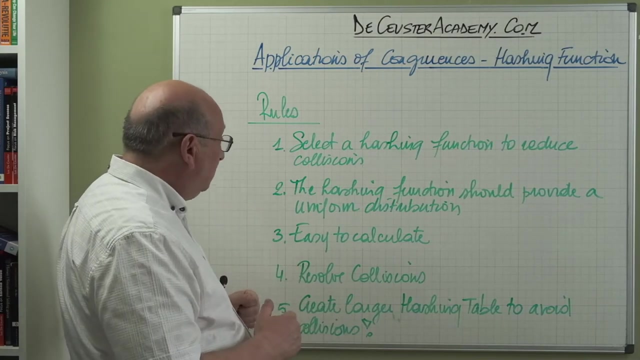 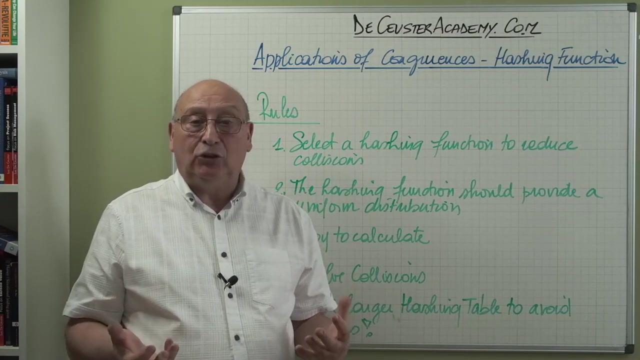 create a hashing table which has more memory space than the total amount of data that we want to put in there. a proportion- seventy percent- would be, let's say, perfect. we have seventy data items and we have 100 memory spaces. but let's have a look in the next part, what we learned in this video and summarize the things we've. 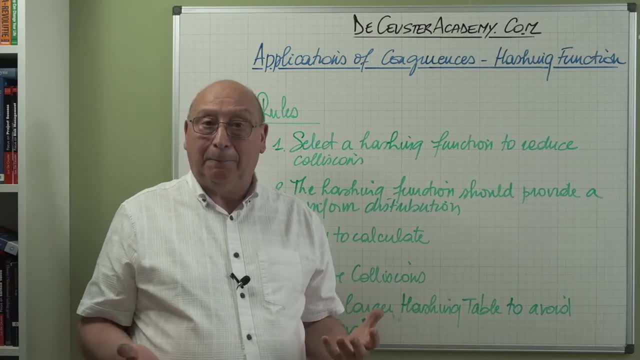 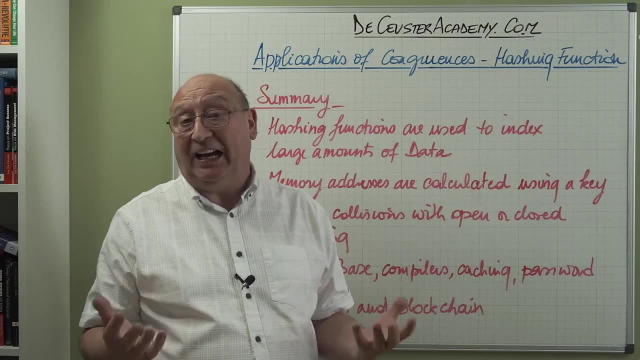 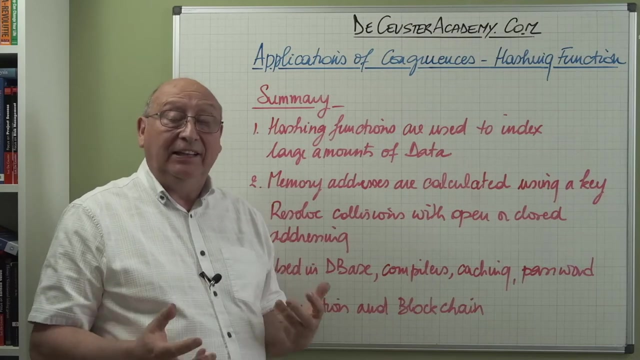 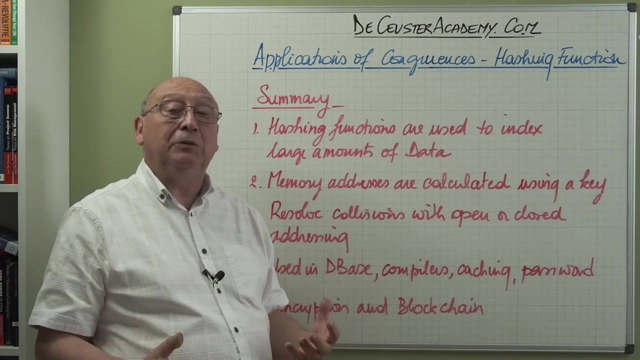 seen the important things about hashing. let us summarize all the important things about hashing and where we can use hashing or where hashing is used first of all. hashing is, or hashing functions are used to index large amounts of data, to allocate them to a specific location, specific memory location, so that they 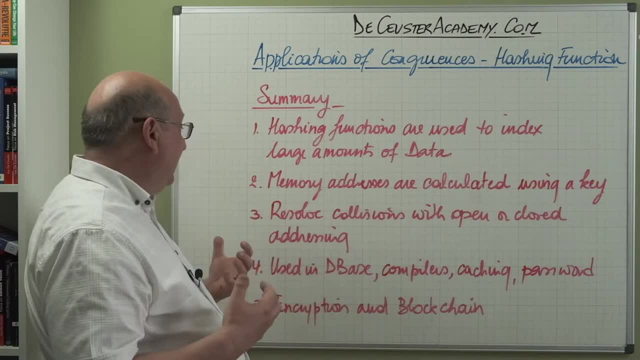 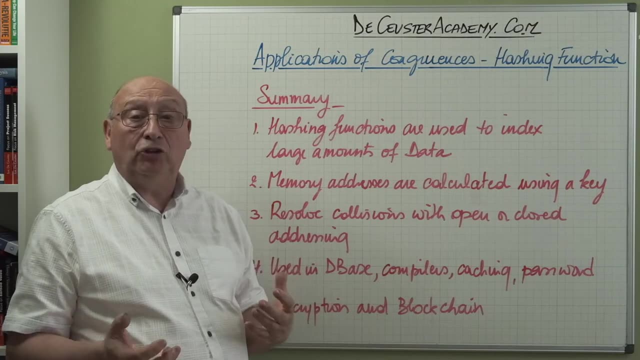 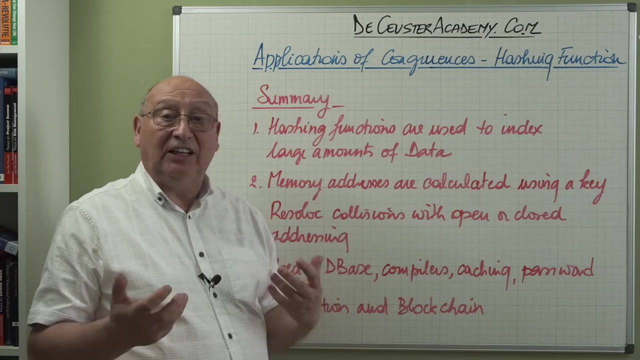 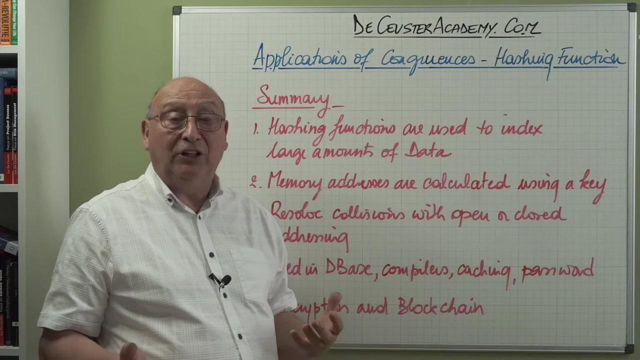 can be found back very quickly and very easily. we calculate the memory addresses by applying the hashing function on a numerical key. when we had data strings, we could transform those data strings in numbers using ASCII. the ASCII codes of every character that we have in the computer, even spaces and everything can give you or will give. 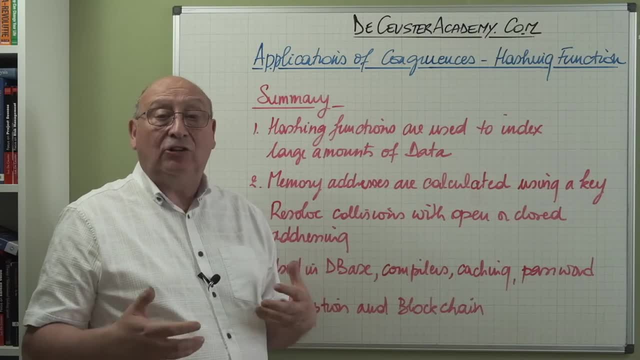 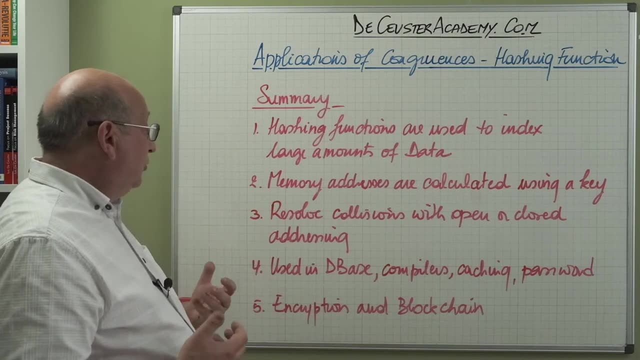 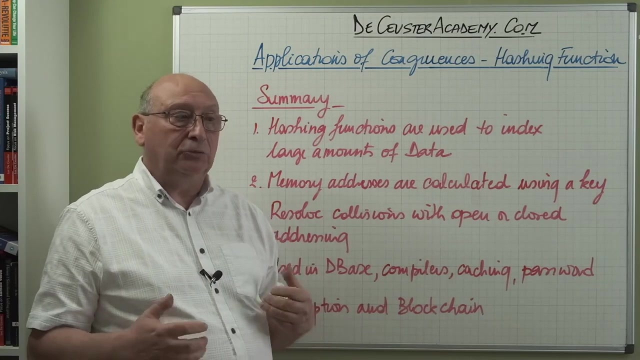 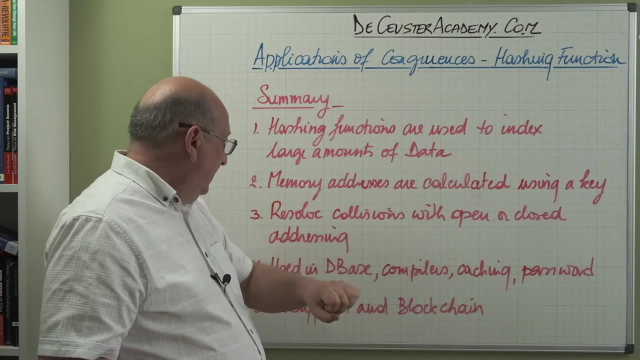 you a number and we can create a unique number for every string. we have to look at collisions. how will we resolve collisions? we didn't discuss the methods to resolve collisions, but basically there are two ways to resolve collisions. we have open and closed addressing. open addressing is what we used before, so we 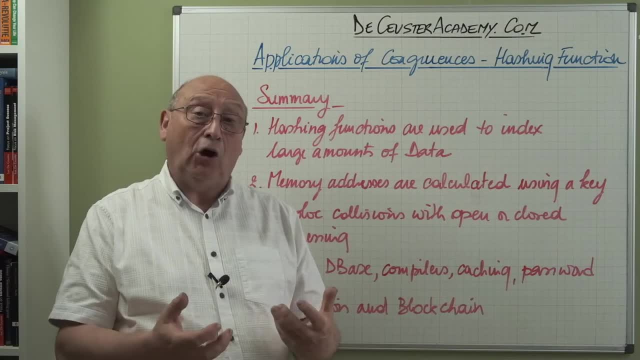 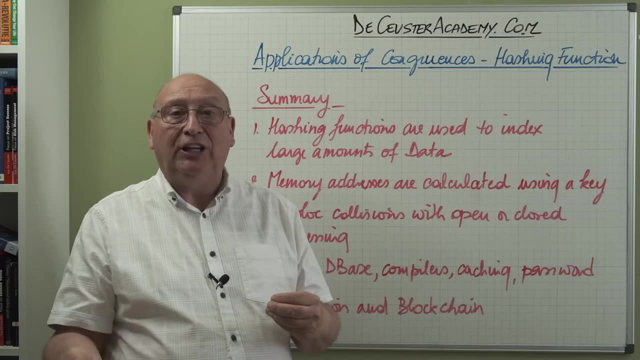 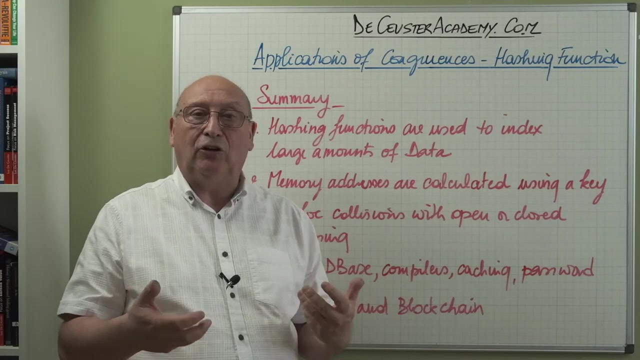 found a memory location that was already occupied, so we went to the next or some other memory location and we continued till we found a free memory location. this is not always very interesting when we have a lot of collisions, because when we want to retrieve the data, we have to go through all those steps again. 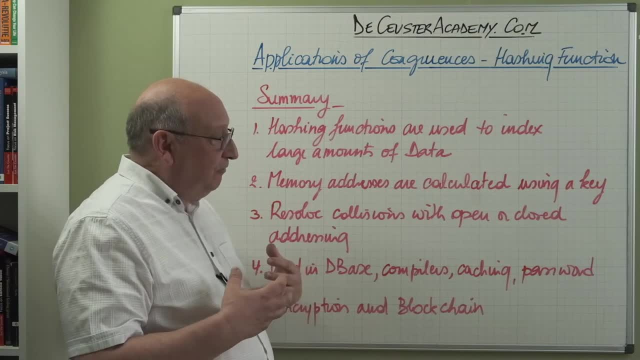 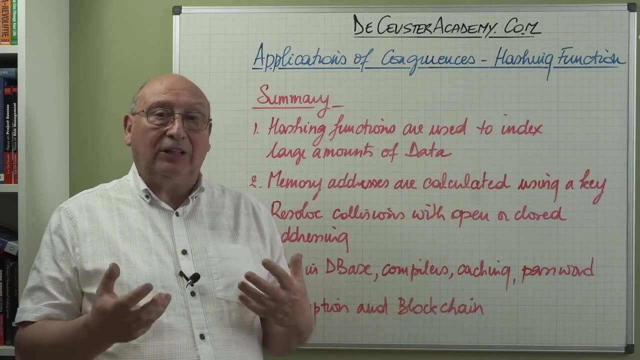 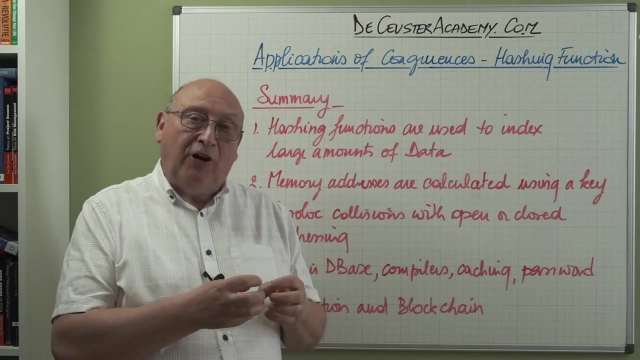 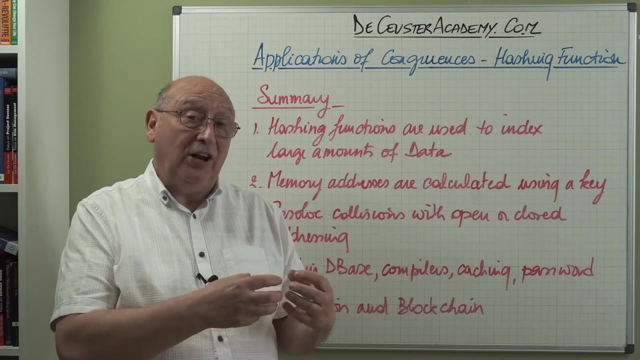 another possibility to find or to resolve collisions is what we call closed addressing. and with closed addressing what we find is whenever we have an occupied memory location, from that memory location with the new data we create a linked list. so every time when we found in our example memory one, we 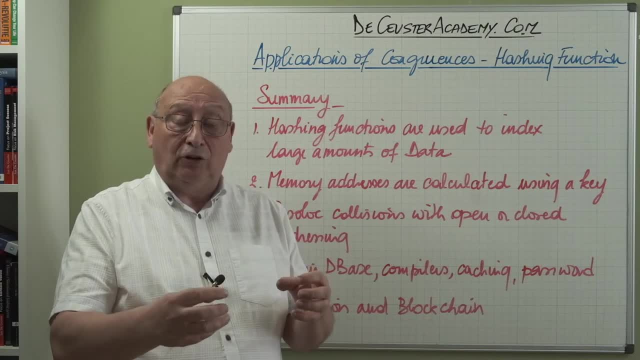 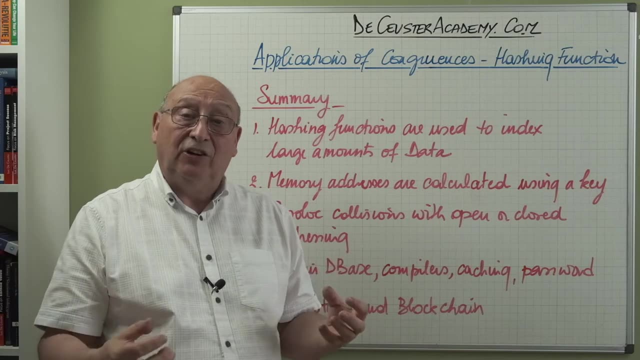 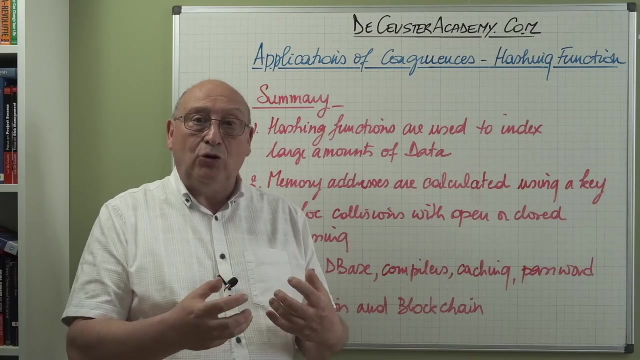 would add one list with the first name, Louie, and then we would add a second linked list with the name Mark. and basically, when we use this method and we find the value, we find the hashing value of the key and the first value is not correct. so we go to the 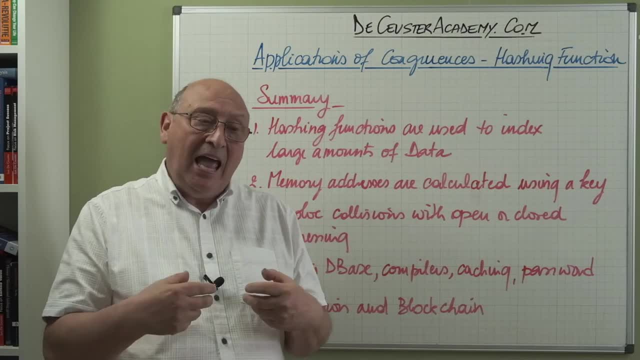 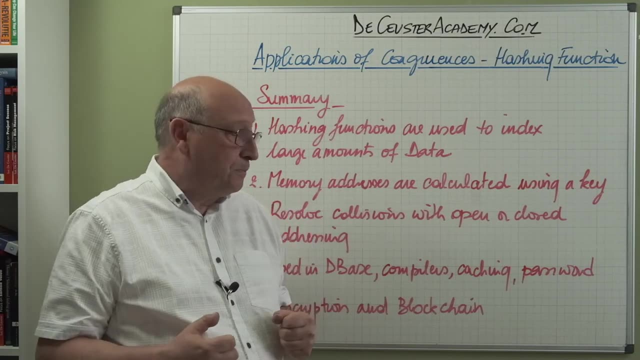 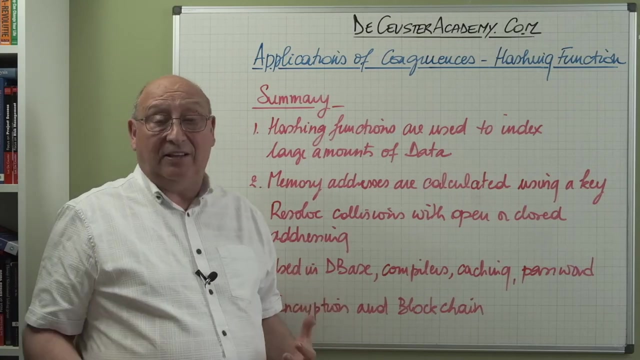 next step in the linked list. so we start looking in the linked list and when we have a lot of collisions, this is a more efficient way of dealing with the collisions. the other things is: where do we use the hashing function? well, we look at D base. indexing databases have very large amount of data, lot, lots of data to 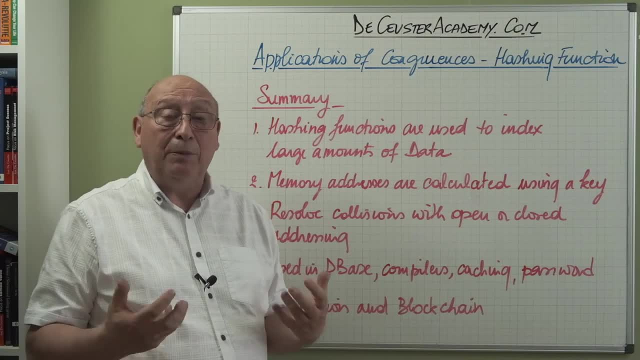 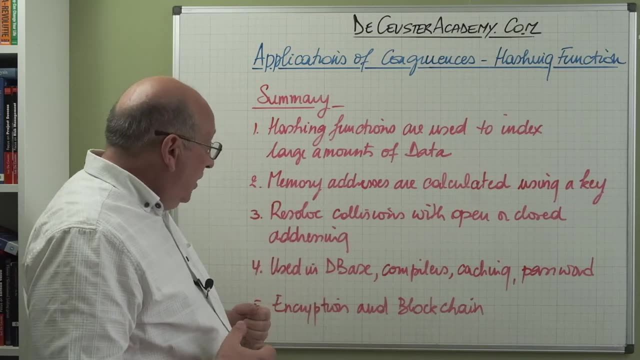 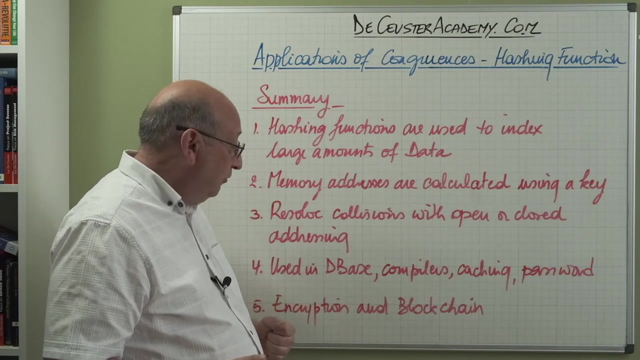 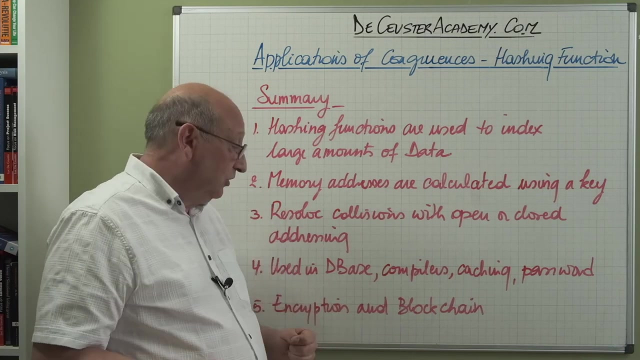 put in memory and we have to put them somewhere. we have to remember where they are. so database indexing is a typical application or the typical way or dip difficult place where we will use the hashing function. we use it in compilers, caching password protections. we can use hashing functions there, but also it's very